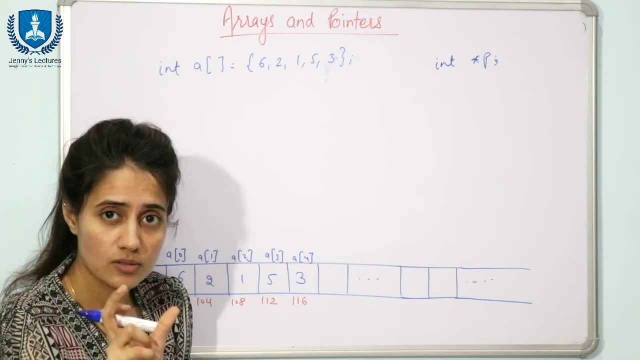 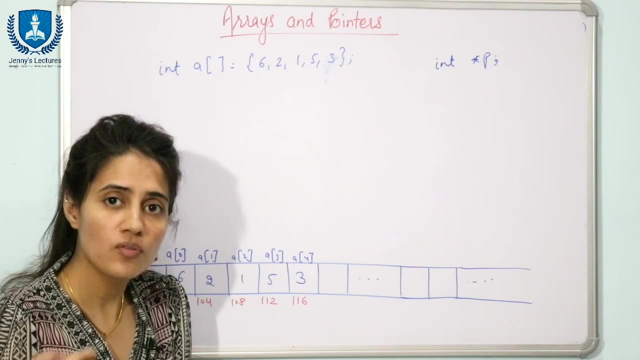 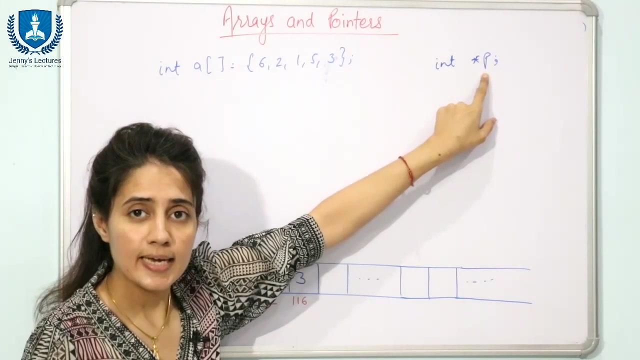 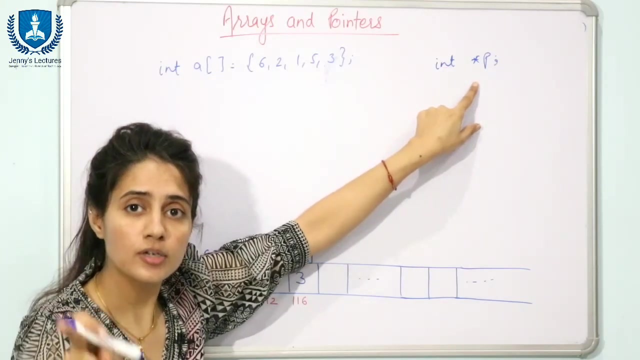 The address of another variable address. So pointer always stores address of another variable and address is always in the form of hexadecimal form. It's a long hexadecimal number. So here you can say this: pointer p contains address of a variable, Fine, And the data type of that variable is integer. So it is a pointer to integer. It is not an integer pointer. Same if you write float. 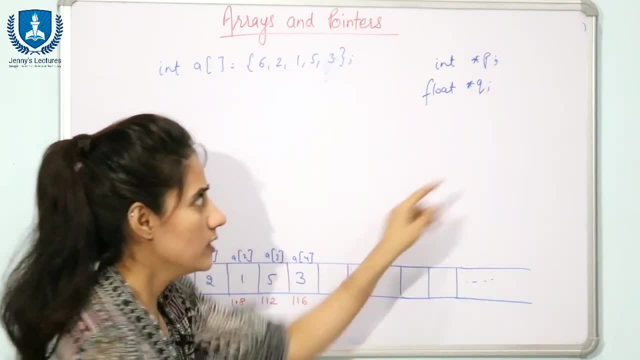 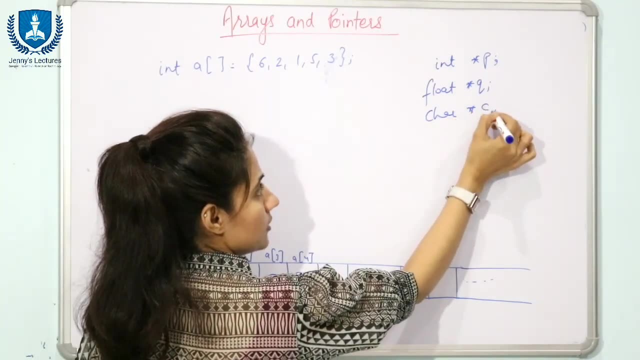 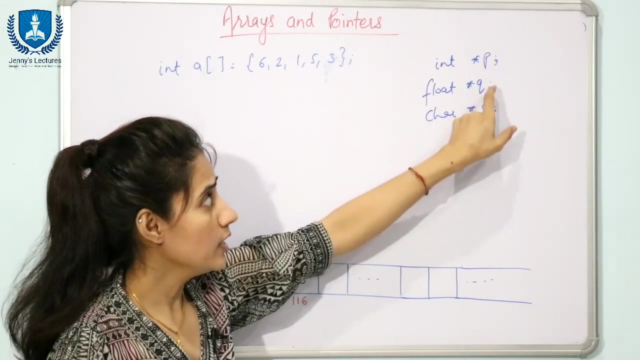 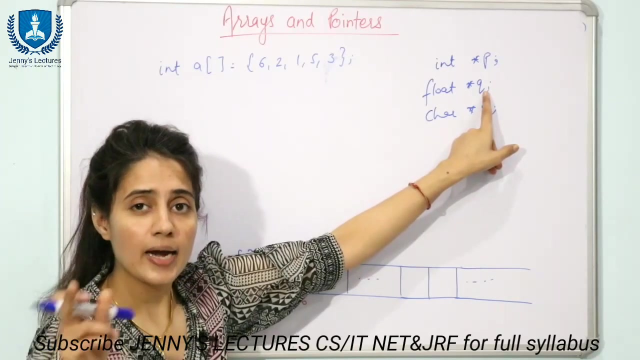 Star, Suppose, pointer name is q, So here you can say it is a pointer to float. If you write char star, Suppose, I am writing c here, So you can say it c is a pointer to character. And all the cases p, q and c, All the three pointer variables will store address. It will store address of a variable and the data type of that variable is float. It will store address of a variable and data type of that variable is float. 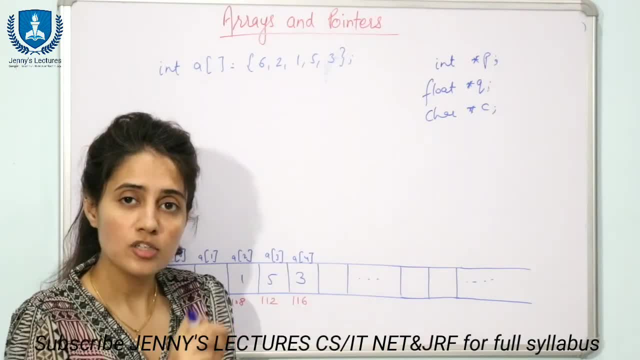 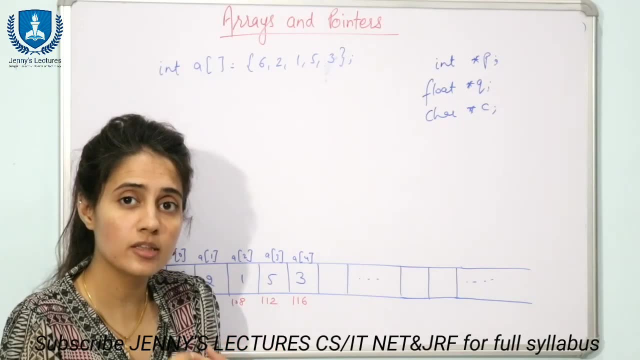 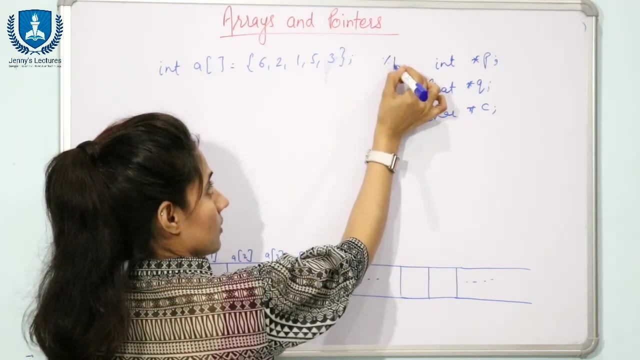 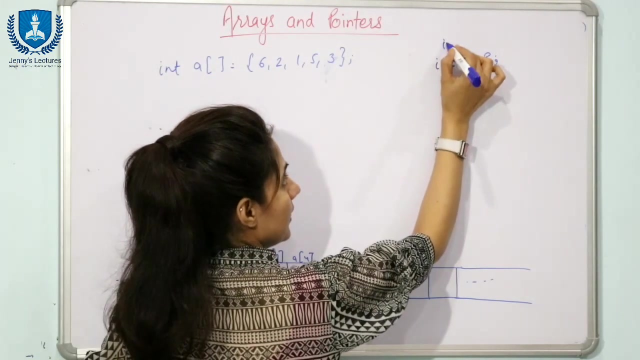 That variable is character Right Pointer is always a long hexadecimal number. If you want to print the pointer, I mean the value of pointer, you can say the value that is stored within that pointer, that address, In hexadecimal form. then you use that percentage p format specifier. Fine, Now see. Now let us take one variable I am taking. suppose int b is equal to 10.. See, this memory is a long type of p, So b is equal to 10.. 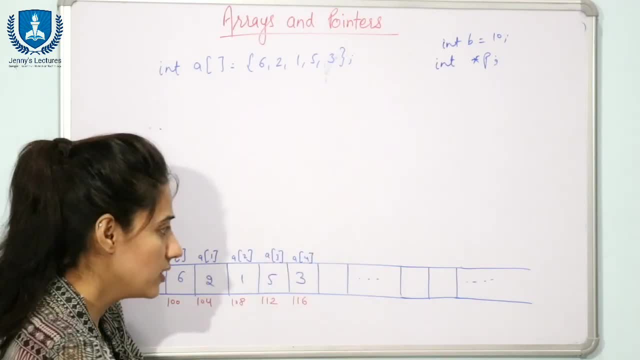 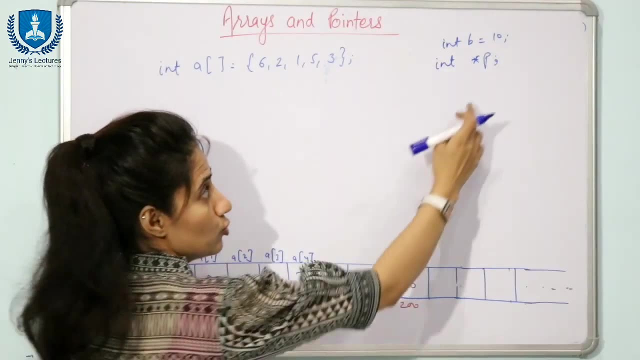 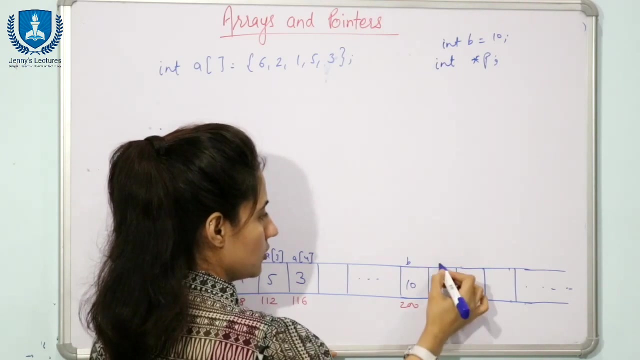 bytes. so these are bytes. every byte is having its own address. so somewhere in the memory, suppose at address 200, this b value has been stored. that is 10, this is b value. so now this for this pointer also. somewhere this pointer is also stored in memory. so let us take this case. here we have this. 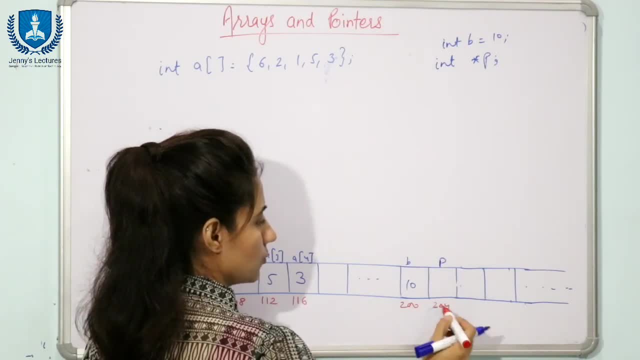 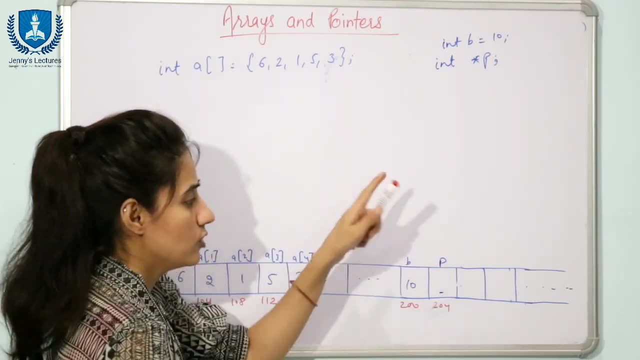 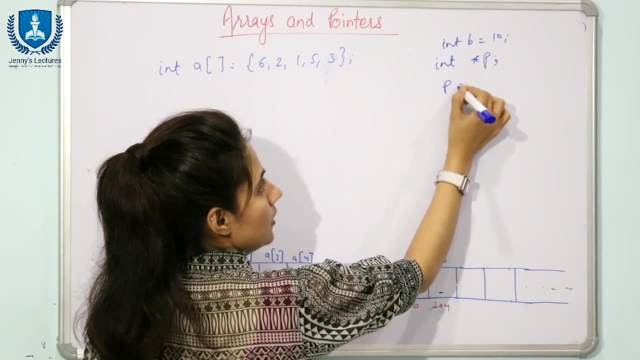 p and address of this p is suppose 204, right, any address you can take in the memory. so what is the value of this p? this value of this p is always address of another variable. so here you can write something like this: p is equal to address of b. you can initialize a pointer something like this: 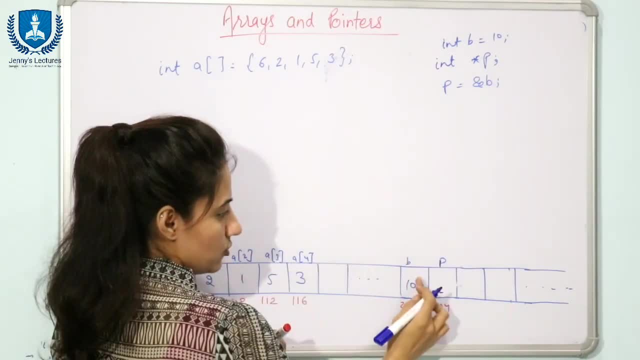 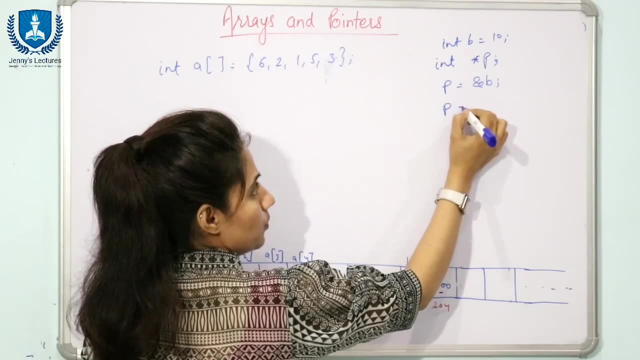 now, what is the value of this p that is address of b. address of b is 200. so here you will write 200, fine, but you cannot write something like this: p is equal to b. in this case, what is the value of this line? the value of b? 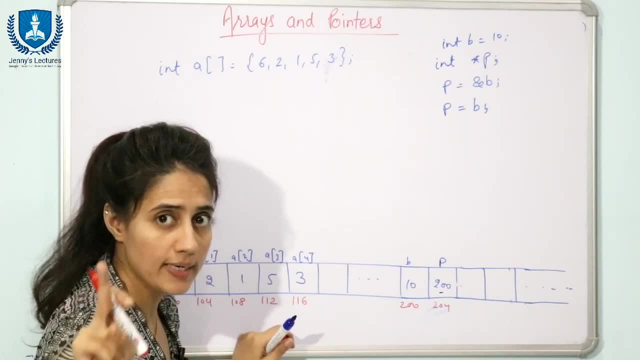 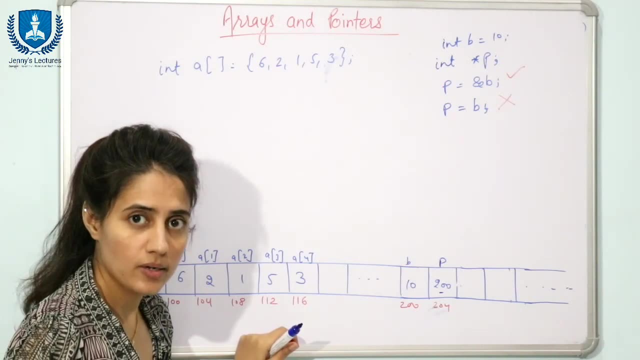 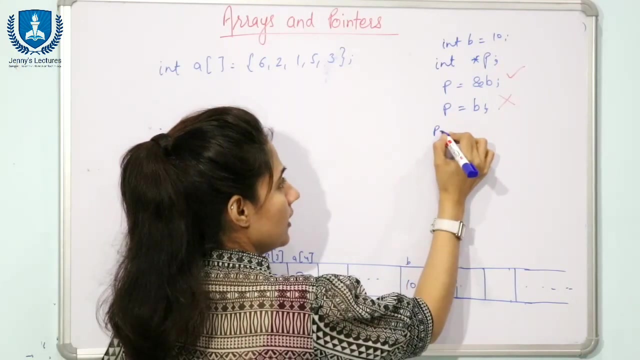 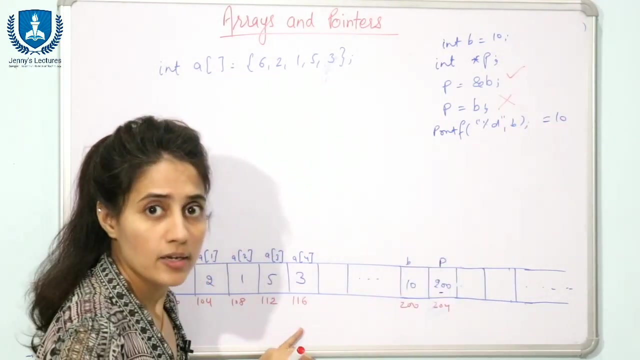 10. 10 would be stored in pointer, but pointer cannot contain a value. it will always store an address, so this is invalid. this is right. fine now if you want to print the value of this b, then simply what what you can print in printf. you can write percentage d and b. the output would be 10 if 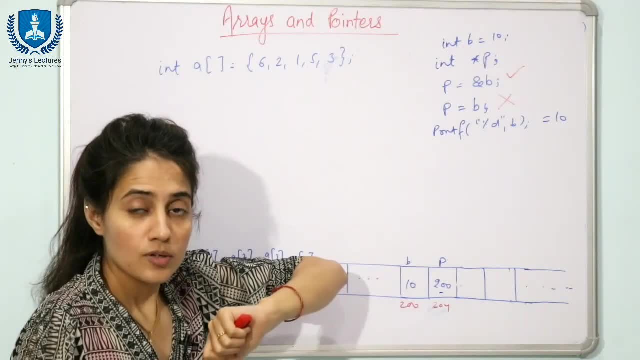 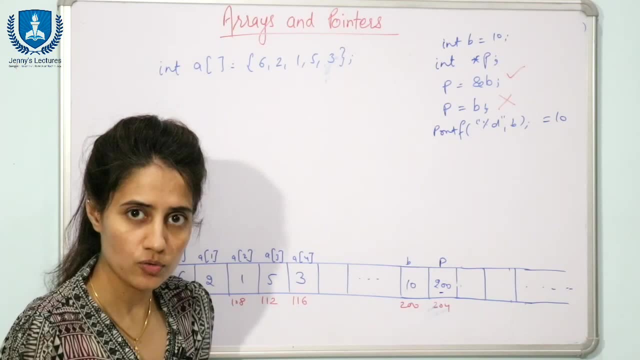 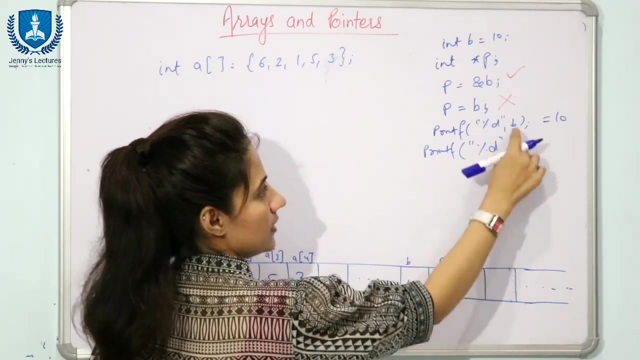 suppose, using pointers, you want to print this value. so how to print? you have to use the value. you can use a d referencing operator, that is asterisk only, star only. you can say: fine, so here what you will write: printf percentage d rather than b. you can write what? because see this p contains 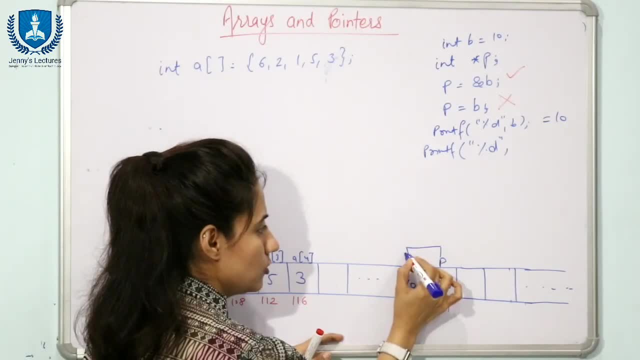 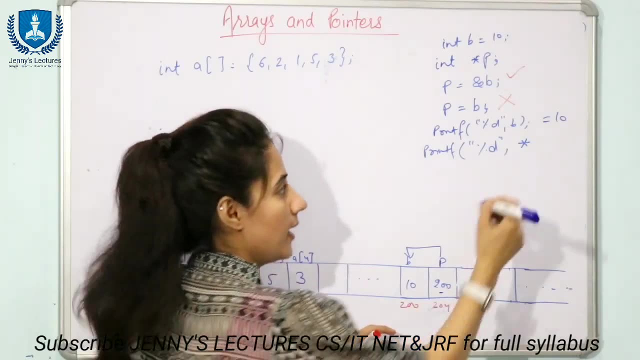 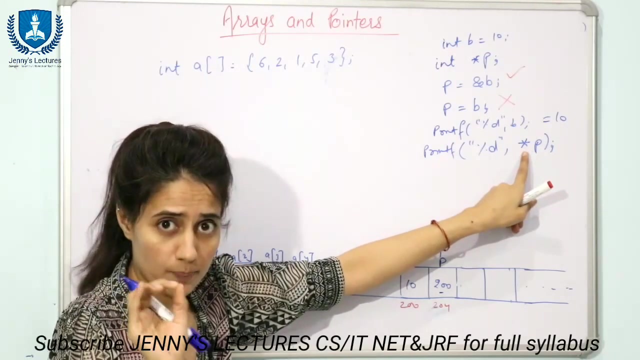 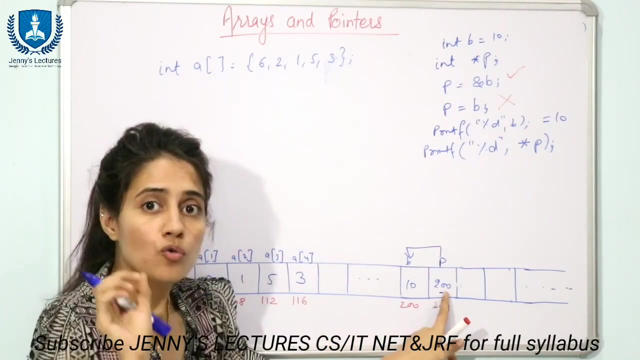 address of b. it means this pointer points to this b. fine, so you will write asterisk and p. you want a entrance of b over b and you are saying, if you press 잘못, what this arbiter will do. you want a whole column. this will print the value and B and then another p will be pe, onder to the. 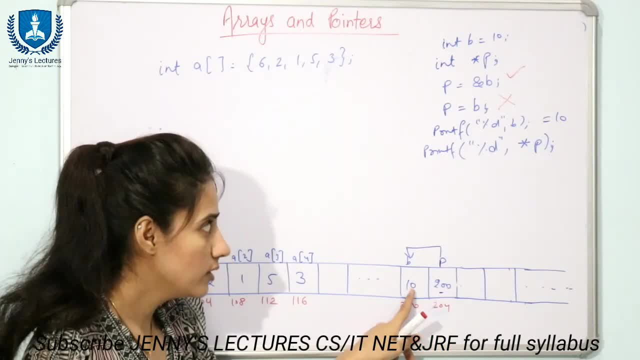 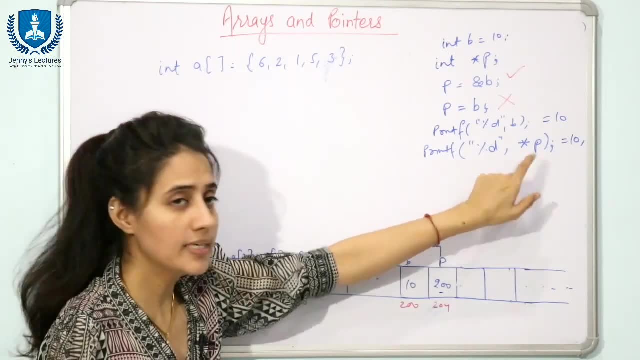 value of this base p is 0. if the value is the word d or the queue consiste in the last five plus term, and this word d means that byight and this comma of 12 and the formula is 100, you have to write the value of five, this point one, point two, point three: anti, terrible option. 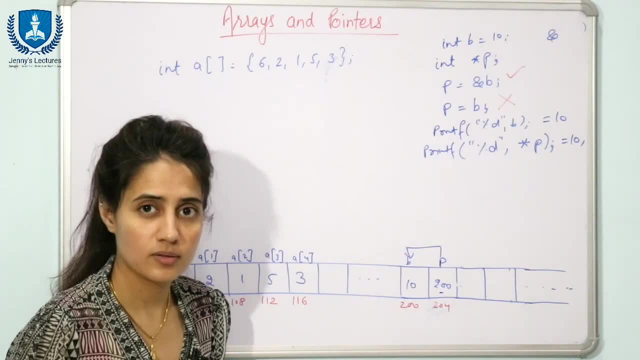 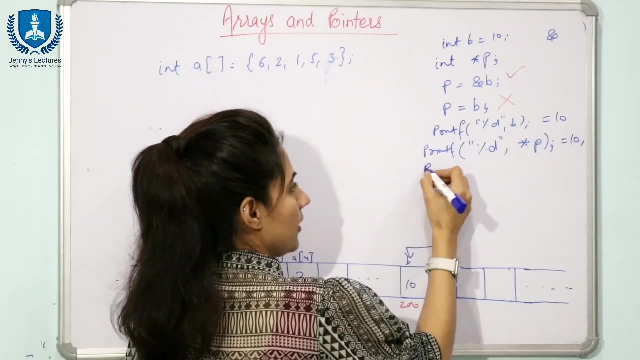 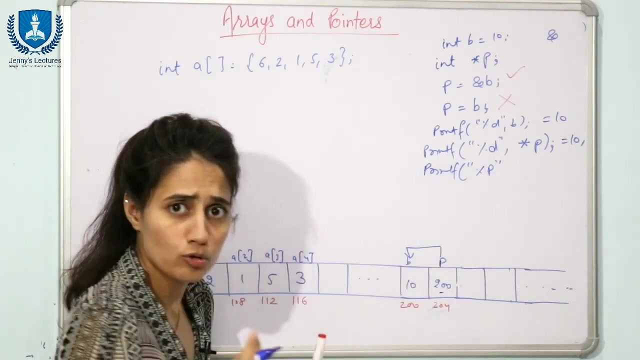 and this is what dereferencing operator: fine. and if you want to print the address of b, so simply in the printf, you can write. if you want to print the address in hexadecimal form, then you will write percentage p. you can also write. percentage x also, you can also write. 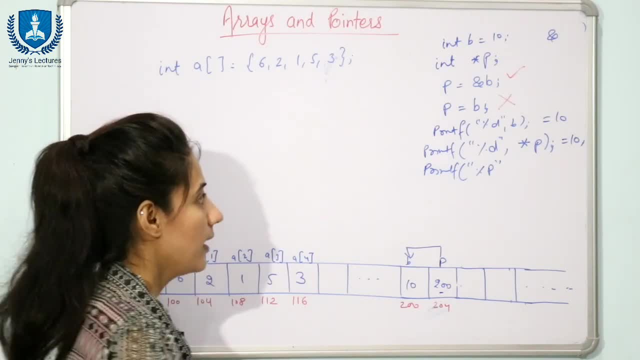 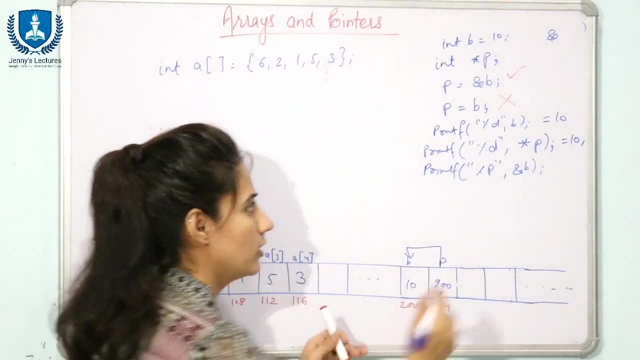 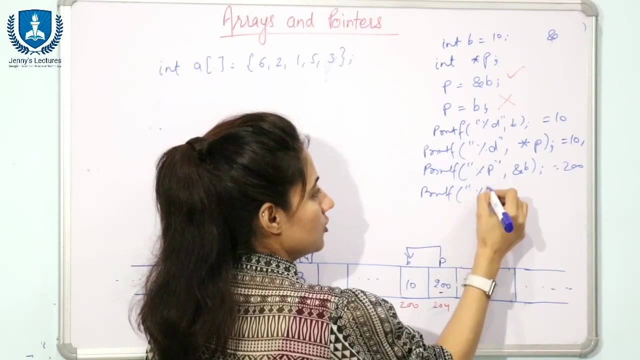 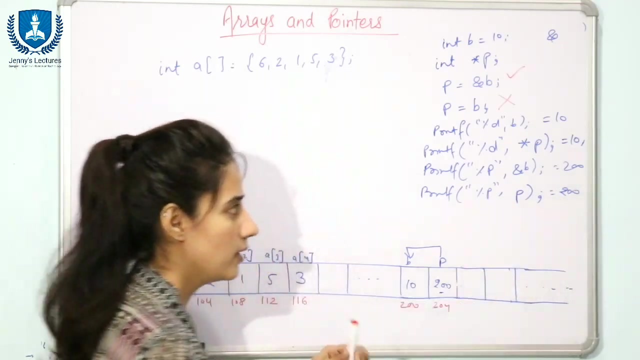 somewhere it is written percentage u, fine, and so you can print address of b. it will print address of b. here i am taking address 200, so it will print 200. and another way of printing the address is what printf percentage? p simply print value of p simply you can write p, it will also print 200. 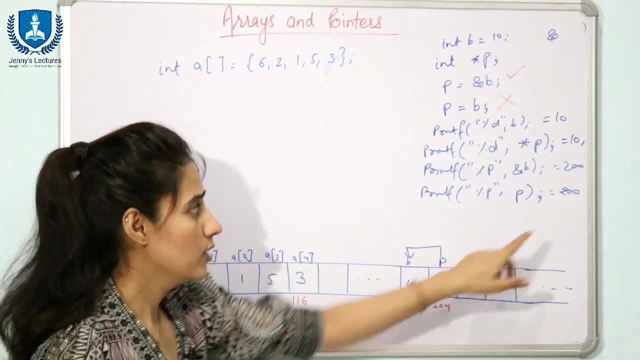 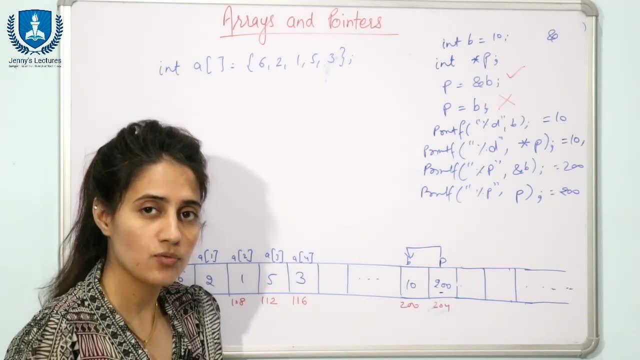 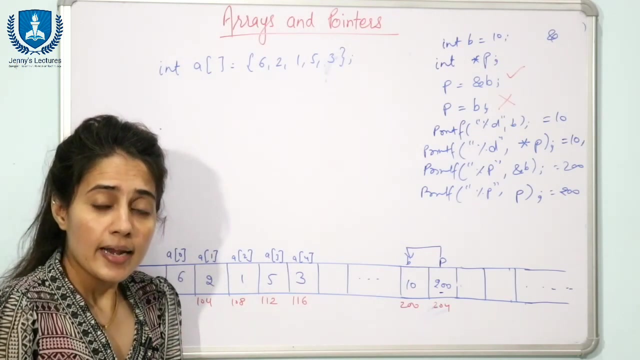 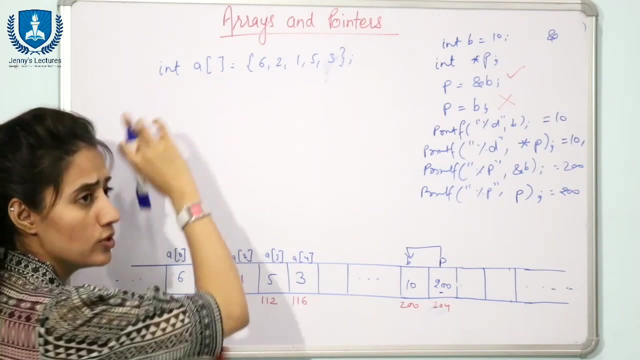 because value at p is what 200, that is address of b. so it will also print 200. fine. so this is the basics of pointers. in detail we will discuss when we are going to discuss the pointers in c programming. now c, how arrays are related to pointers. array name itself x as a pointer. fine. so if you simply print, 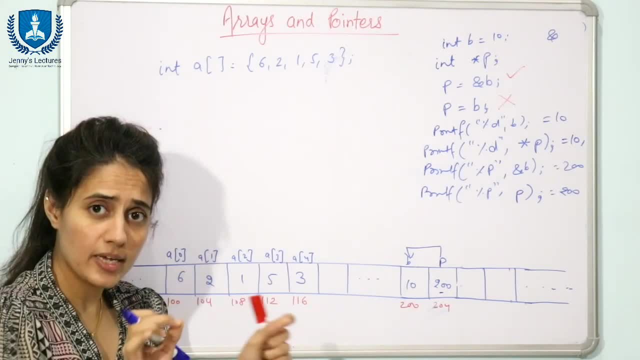 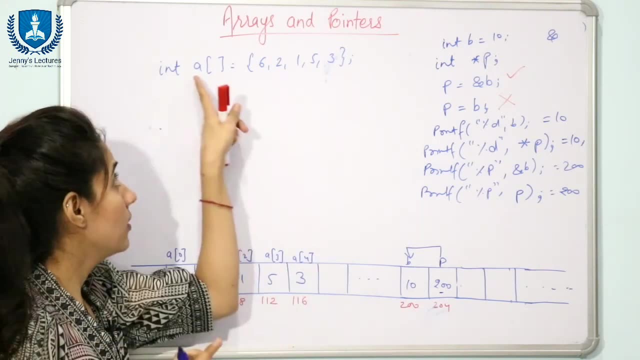 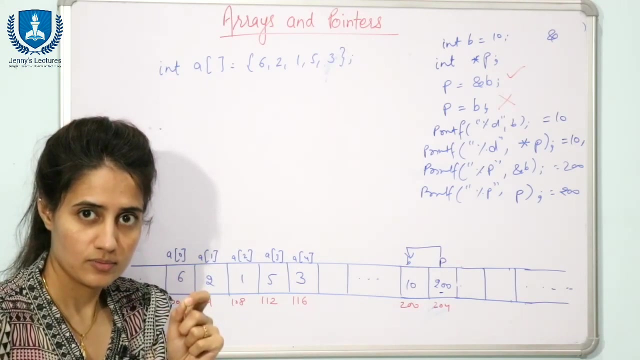 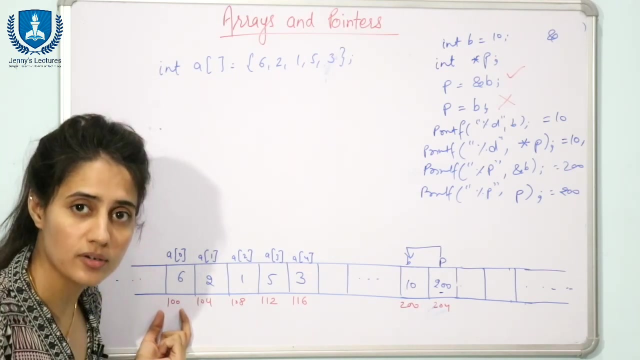 a. i am simply writing a in the printf. i am simply writing. suppose if you write printf: percentage p, simple print a, the array name a, then what should be the output? it will print the base address of the array. it will print. here i am taking base address 100, so it will print 100. so array name itself: x as a pointer. 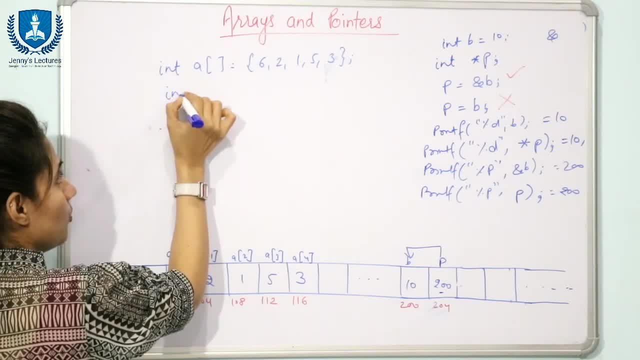 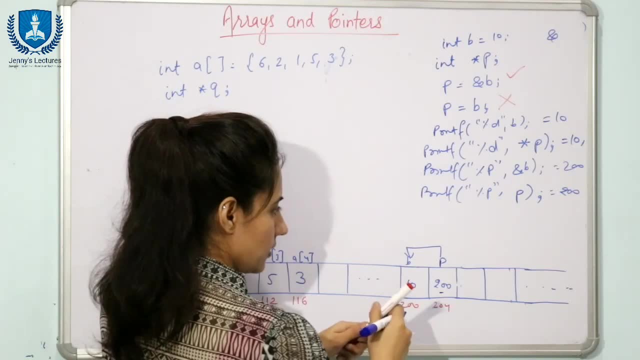 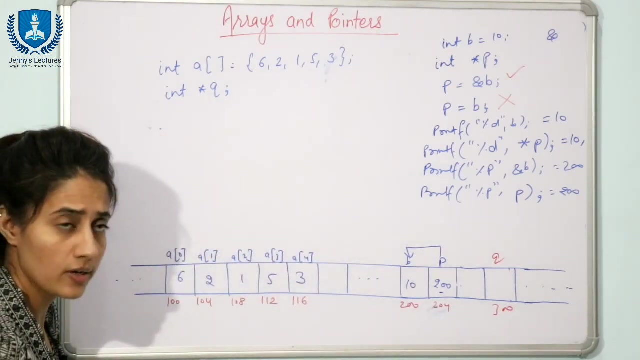 fine. so in this case, in this case, if i am taking another pointer, suppose int star and q in somewhere in memory, suppose here i am taking q, this: this is allocated to q at address 300, suppose fine, and have to initialize this pointer now. in this case, 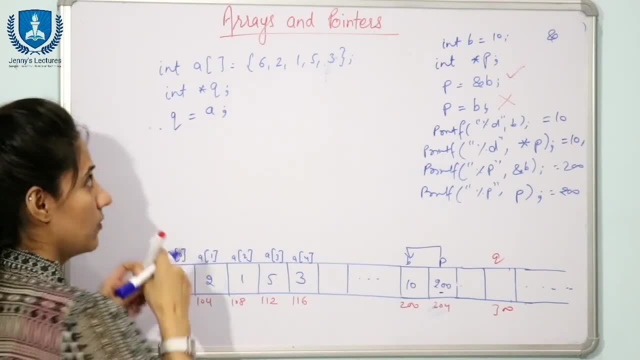 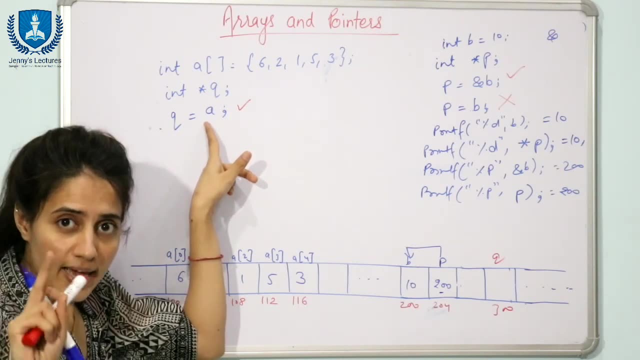 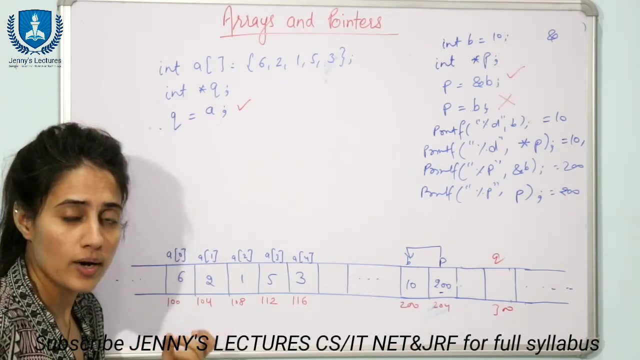 can we write: q is equal to a? yes, you can write. this is correct, but in this case it is not valid. now, in this case, why it is valid? because array a is array name and array name always contains the base address of array. so this 100 would be assigned to q and that is fine, because q is a. 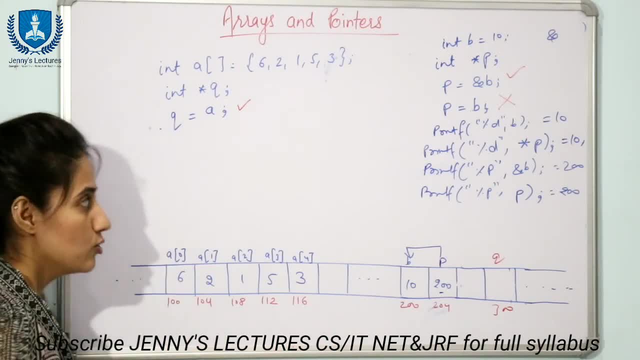 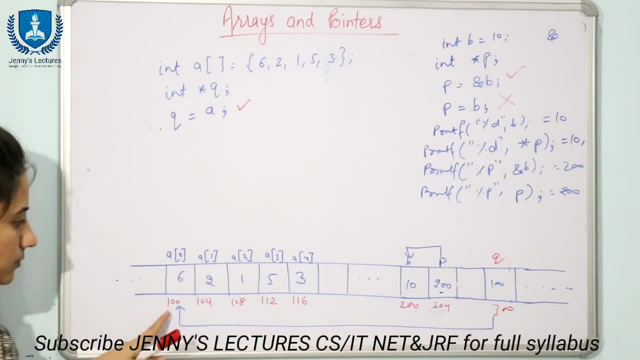 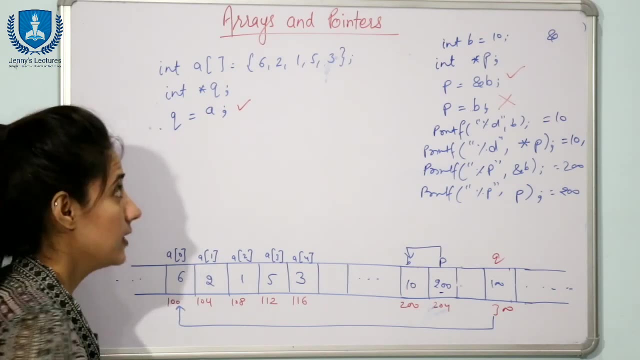 pointer and that will contain address of another variable. so here in the q, what value is to be stored? 100, so this q would point to here. so this q would point to here, so this q would point to here, this address of that element at zeroth location. fine, see, that is also correct. if now, if you write, 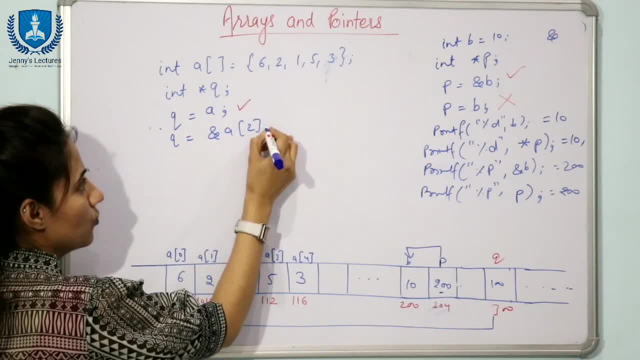 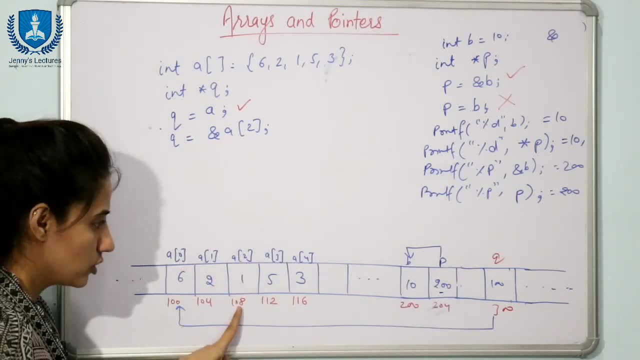 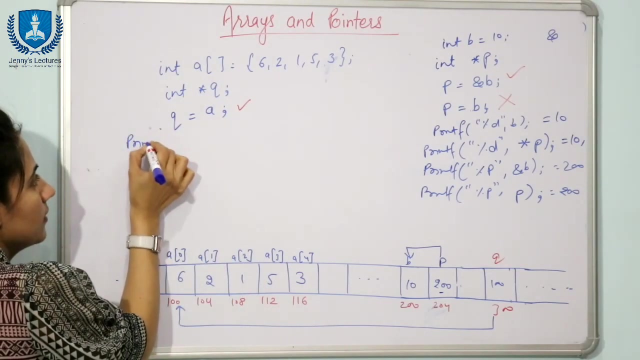 q is equal to address of a of 2.. now this pointer will point to a of two. a of two means this one address is one zero eight. now this pointer will points to one zero eight. so now, in this case, see if you will print %σ and %r. 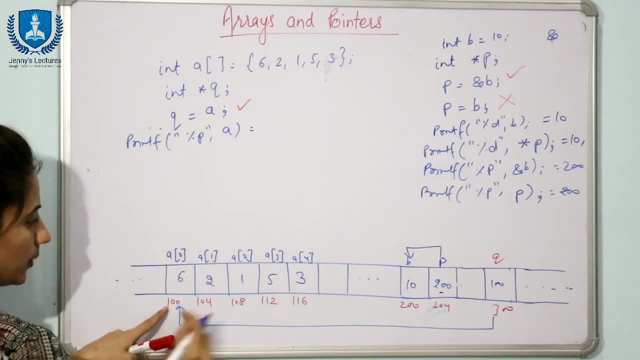 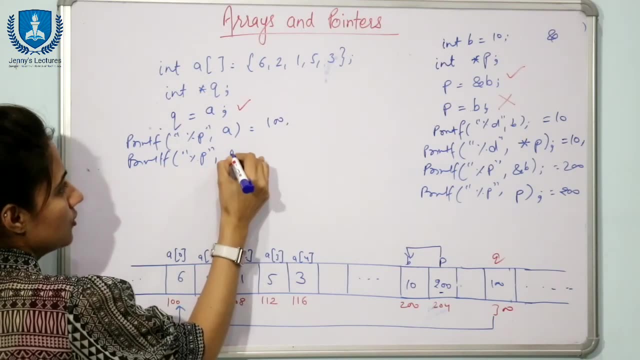 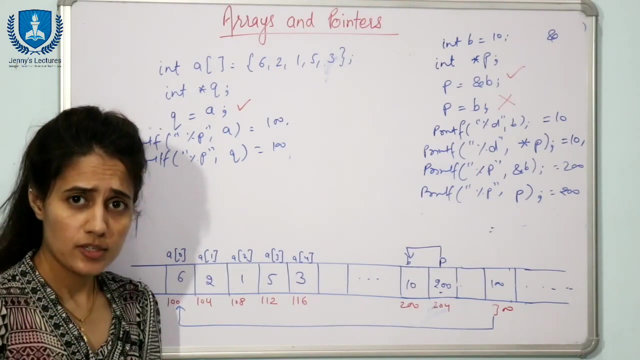 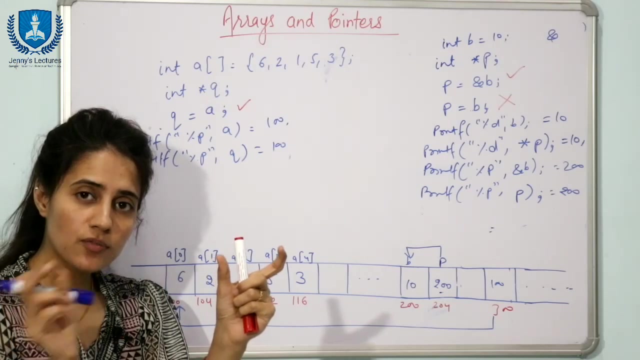 p and a, then it will print 100. fine, and if you print %p, this q, it will also print 100. q is also 100. next thing about pointer is you can increment a pointer and decrement a pointer. pointer contains an address, so you can add some integer value in address you. 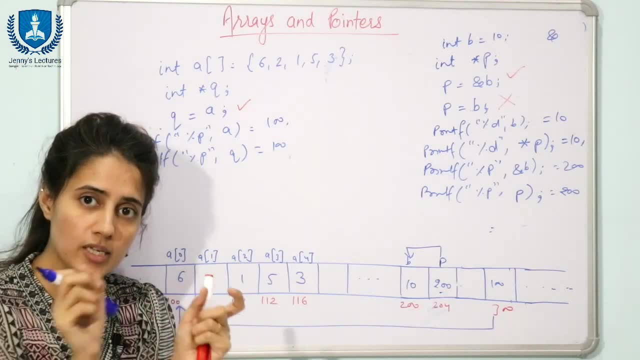 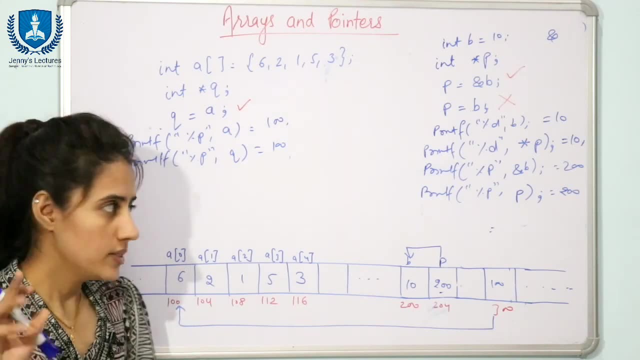 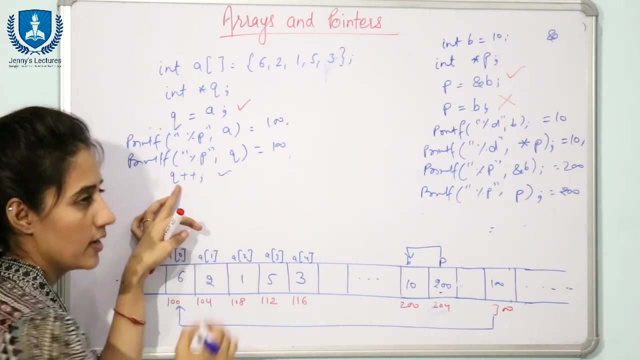 can subtract some integer value from address, that is allowed. but address plus address is not allowed. address into address is also not allowed. fine, see, in this case, in this case, if i write now q++, that is valid, q is a pointer. now the value of q is what say? here we are. 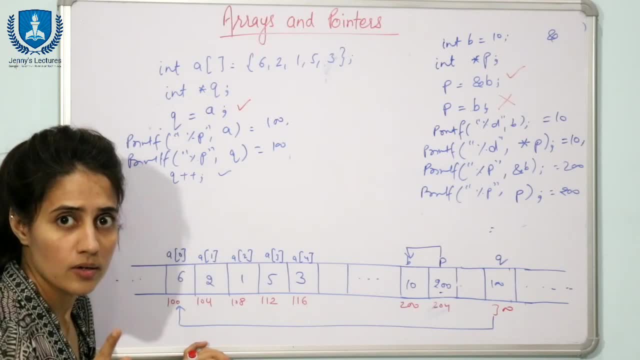 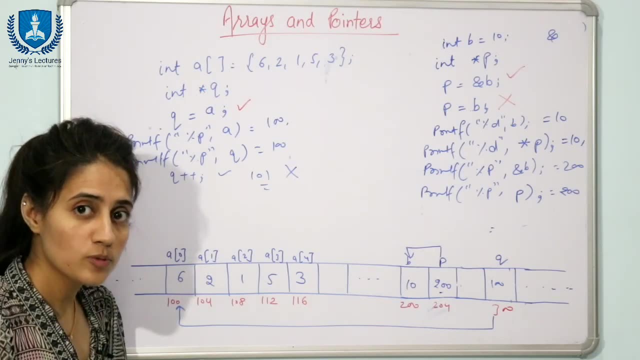 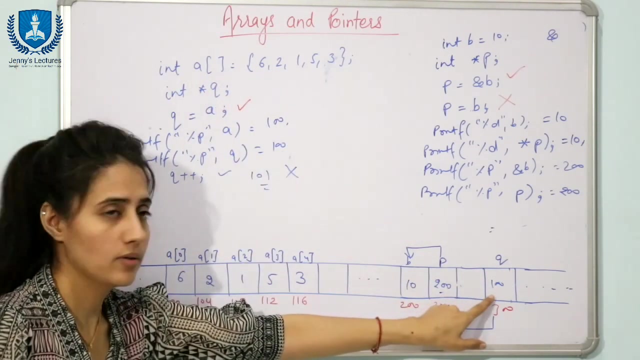 taking this q: fine, so value of q is 100. but if you say it will becomes 101, that is valid. that is not true. so now q++ is what see? now q contains address of another variable, that is integer variable. int. integer variable- fine, so that is why if you do q++, then it will. 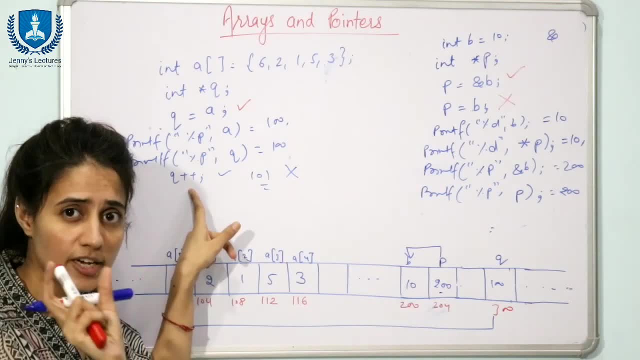 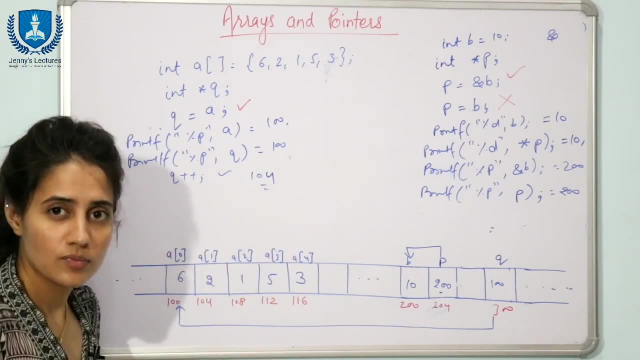 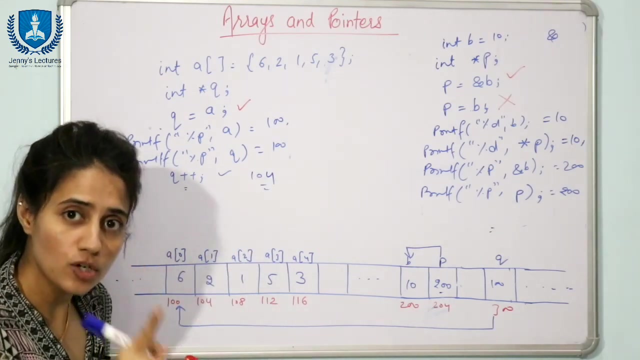 increase by how many bytes that size of that integer? size of integer is 4 bytes. so now q++ becomes 104. now if it is a character pointer, then in that case you can say: if you want, if value of q is 100, then in character pointer it will increased by 1, that is 101, because 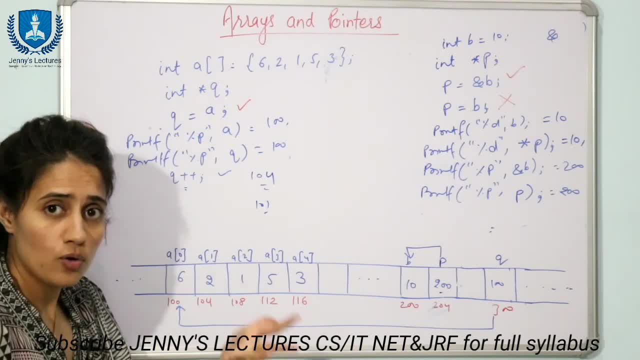 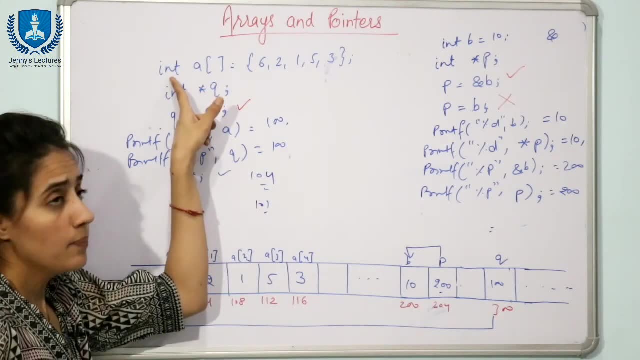 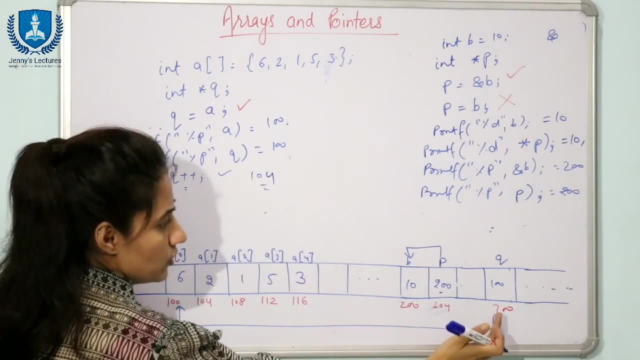 character will take 1 byte right in float. it would be incremented by some other factor in double it would be incremented by some other factor in that factor is what? the data type, the, that size of that data type. fine, now see, if you do q++ now this q would point. 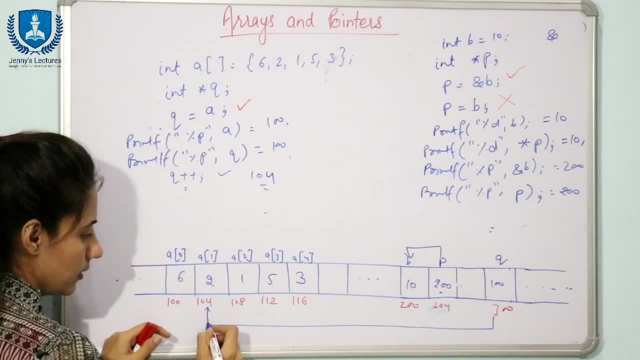 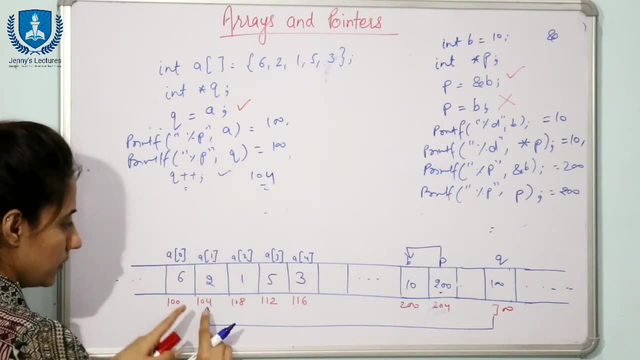 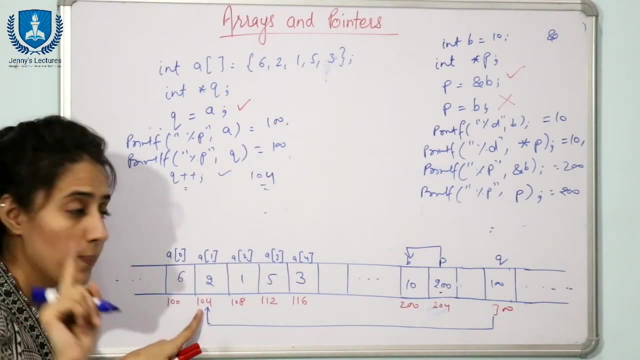 here, not here now. q would point here. Now. if you will print this q, if you will print after this line this q, then the output would be 104, and if you print a again, then output would be 100. but a++ is not allowed. 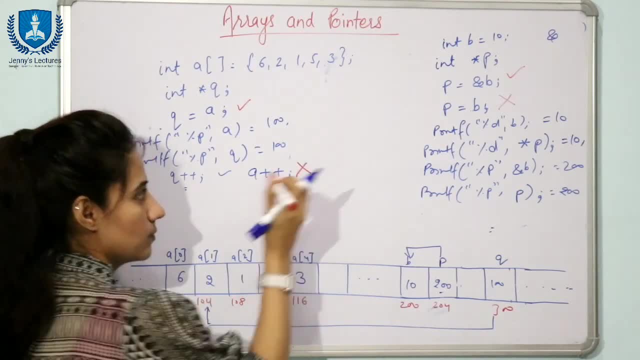 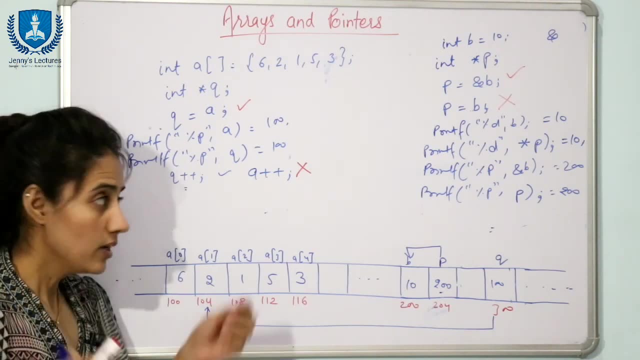 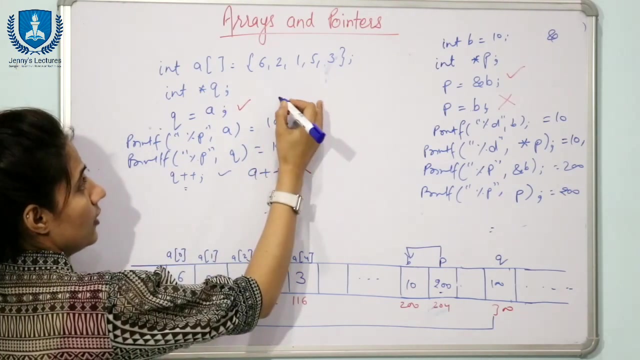 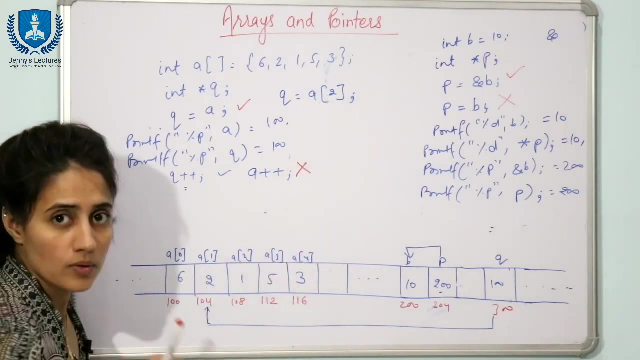 if you do a++, that is not allowed. you cannot change the base address of array. fine, so a++ is not a valid operation, but q++ is valid. you can increment or decrement a pointer. one more thing: if you write here: q is equal to array of 2, is it valid? no, because array of 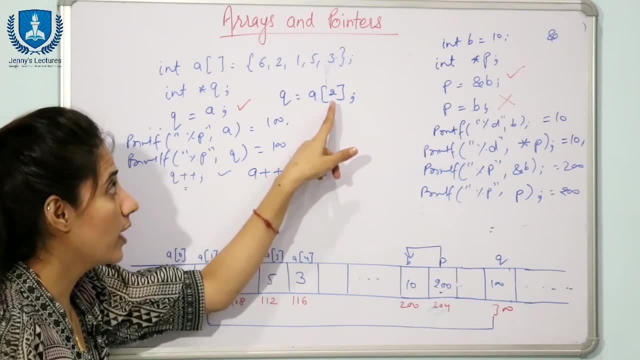 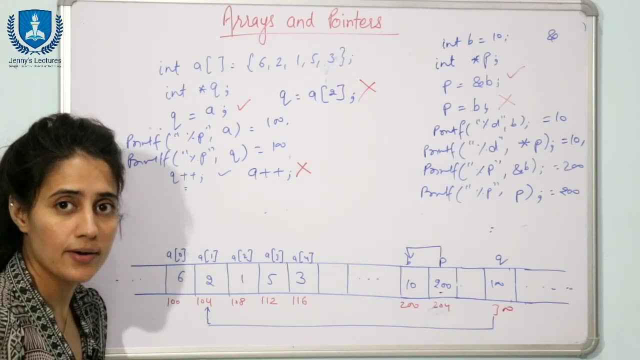 2 means we are we are accessing the value that is stored at 2, that is 1, and we are assigning 1 to q. but that is not allowed because q, always q- is a pointer. it will contain address of another variable. that is not allowed. 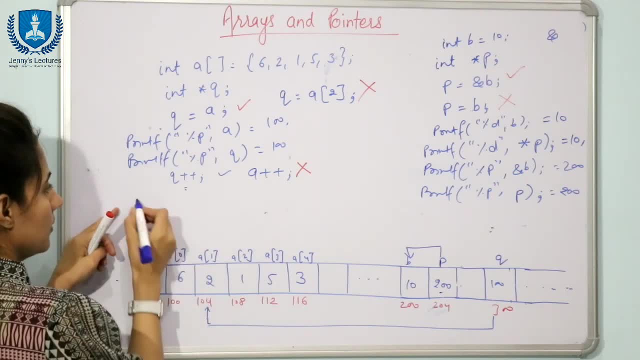 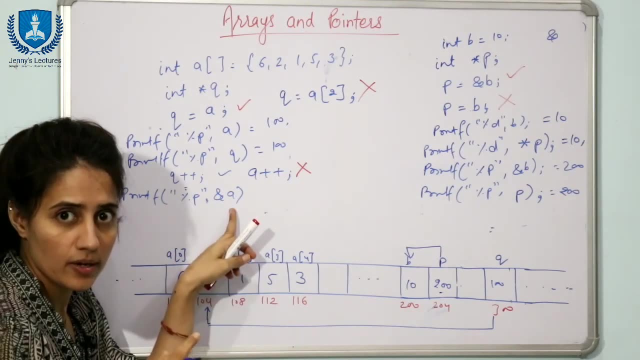 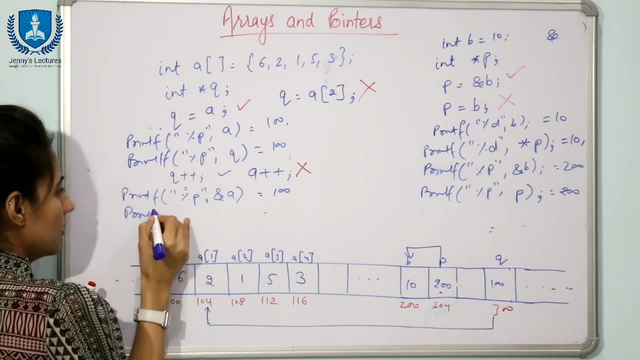 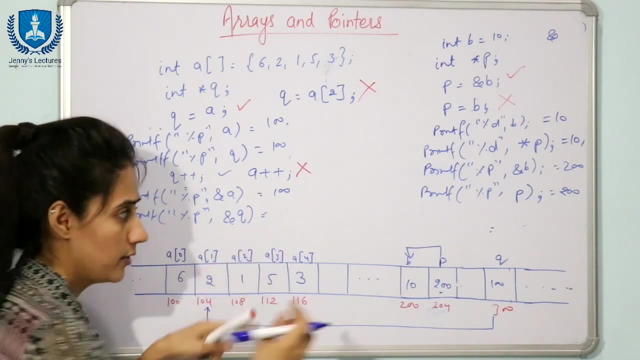 Now the next thing: if you print, see, if you write printf, %p and address of a address of a, it will also print 100 address of a, means that is base address of a. but if you print %p, address of q, so it will print the address of this pointer, the q, address of this q, that 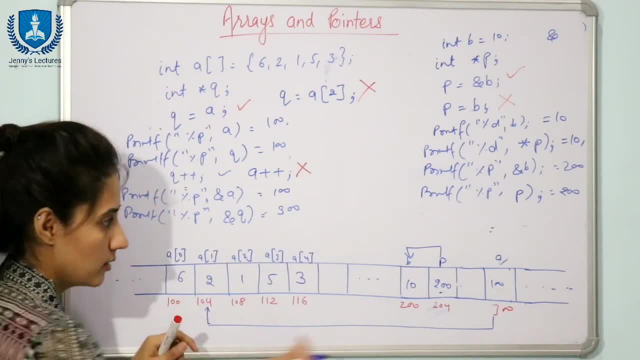 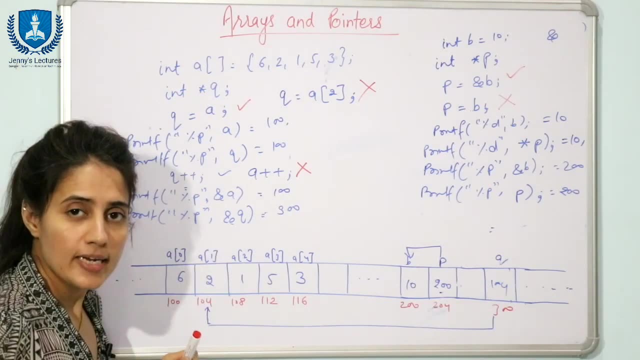 is 300, so it will print 300.. See here: after incrementing the value becomes 104. so in case of arrays you can say: the name of array is equal to address of a. that is fine. a is also 100 and address of a will also. 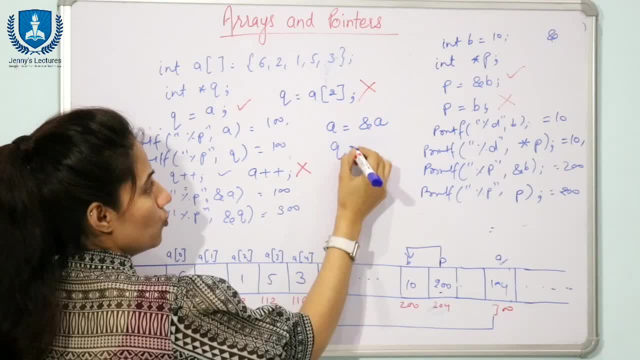 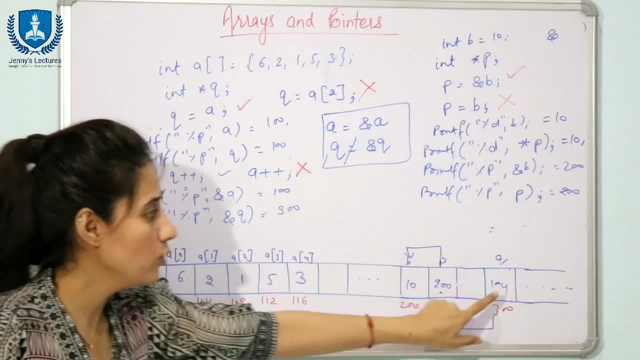 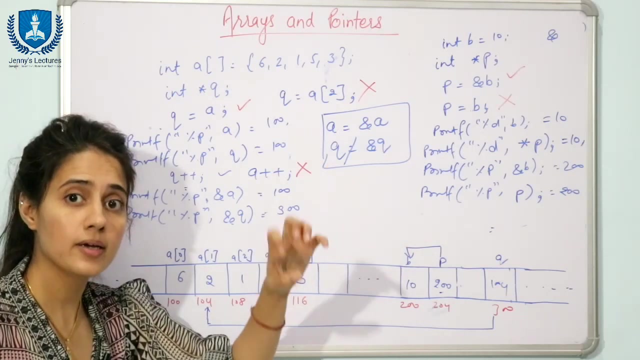 print 100. but in case of pointers, q is not equal to address of q. this thing you have to take care. q will print the value at in this q and address of q print the address of this pointer. But address of a and a is same because a is array. in case of array it is allowed, fine. 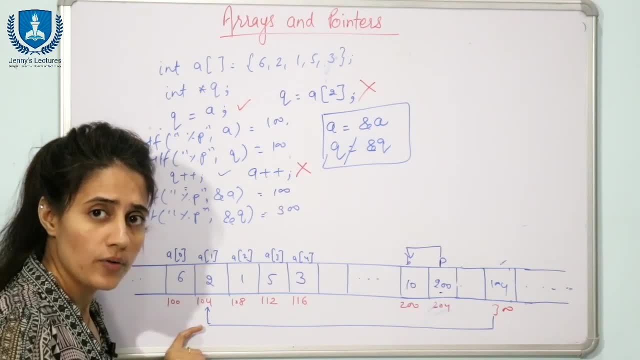 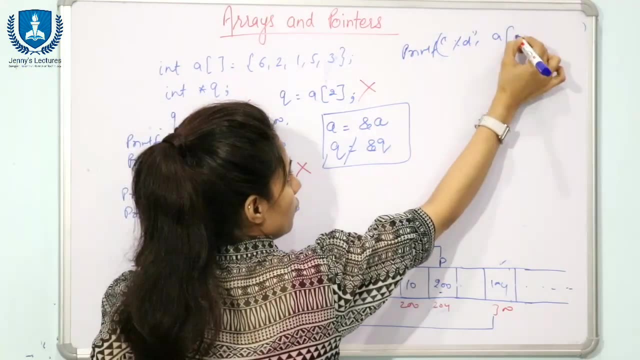 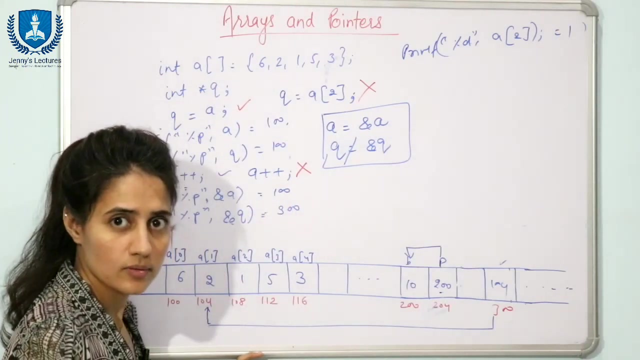 now see if you want to access any element of array, then how you will access. you will write simple printf, %d, and suppose you want to print value at a of 2, so it will print a of 2. that is 1. it will print 1, right? I have told you. array name is itself a pointer. it. 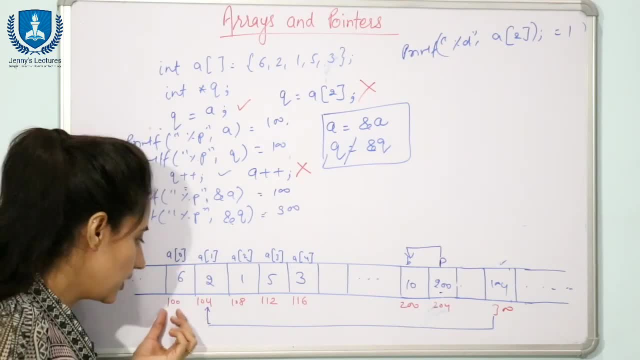 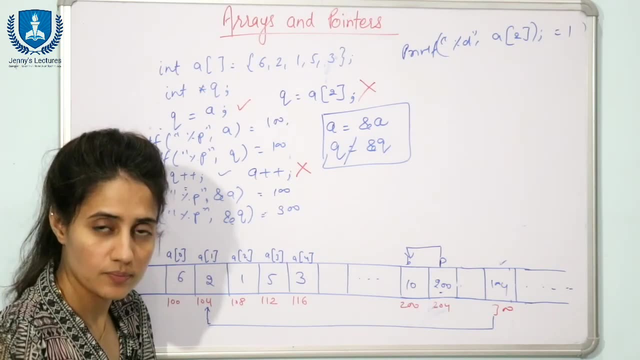 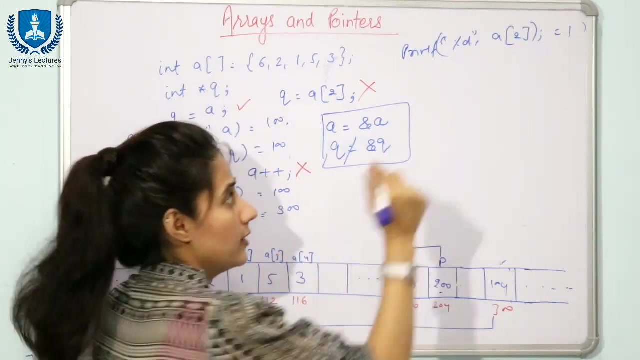 contains the address, base address of the array, and if you want to access values using pointer, then you use what d referencing operator, that is star s trick operator. fine, so in another word, rather than this, what you can write see, this is what see. a will give this 100 base. 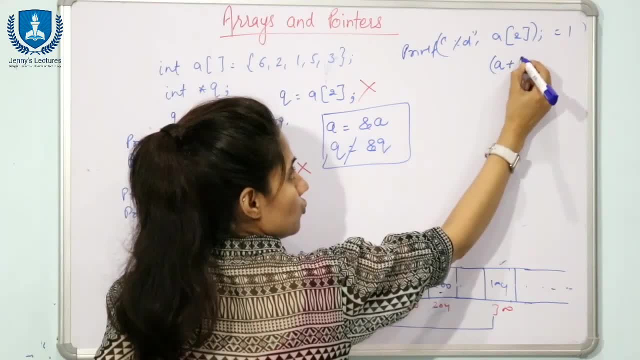 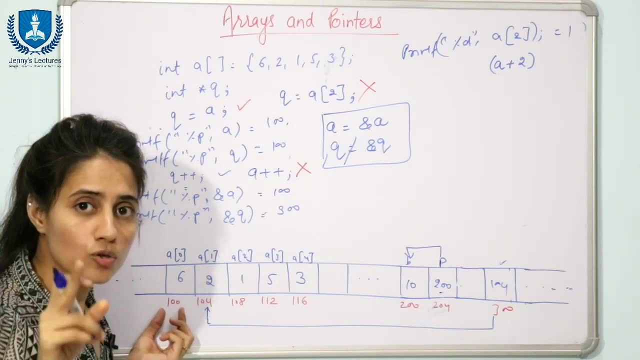 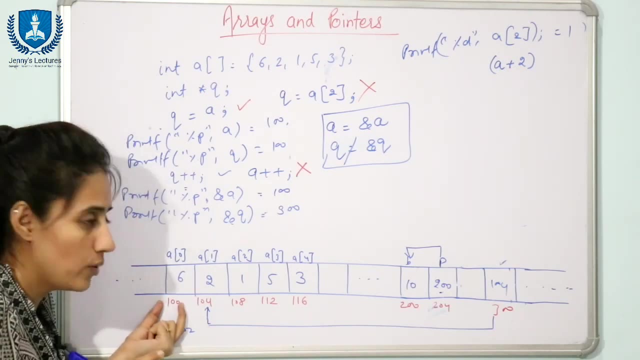 address of array plus. if I do plus 2, it means in base address. in this base address it will give this address. in this address address you are adding what 2 it is. it does not mean that 102. no, I have told you in address. if you want to add, then it will add the according. 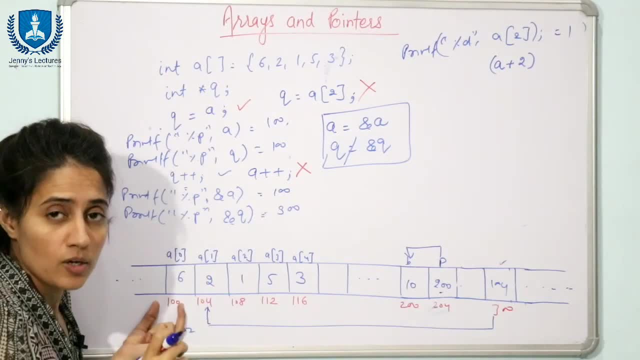 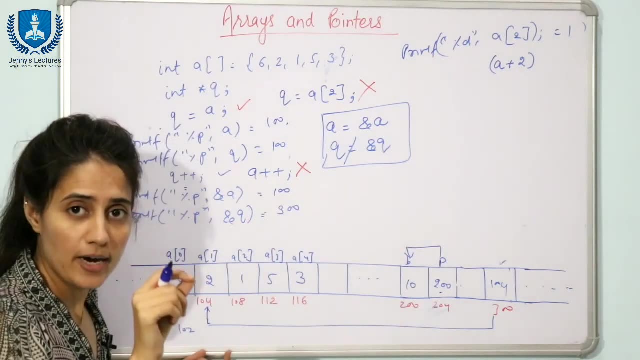 to the size of that data type you are using. so one integer will take 4 bytes and 2 will take 8 bytes, so it will add 8 bytes. it means 108. it means 108 a plus 2 is 108 and if you 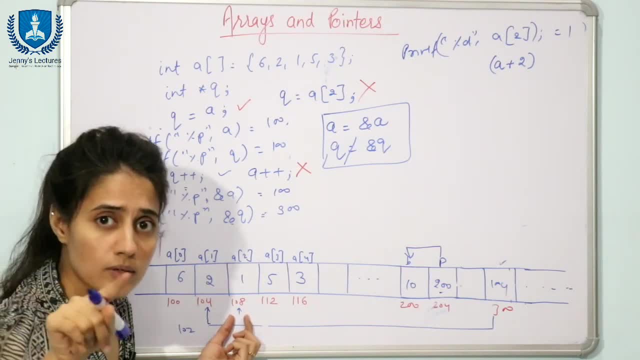 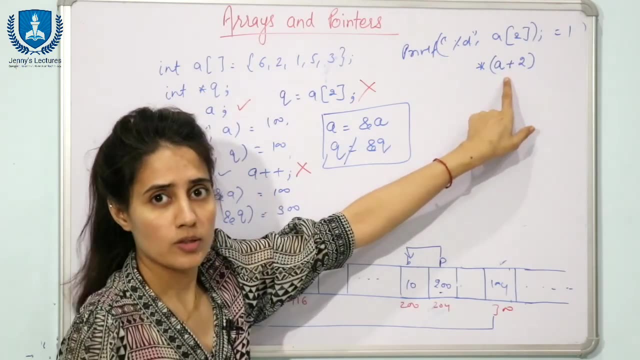 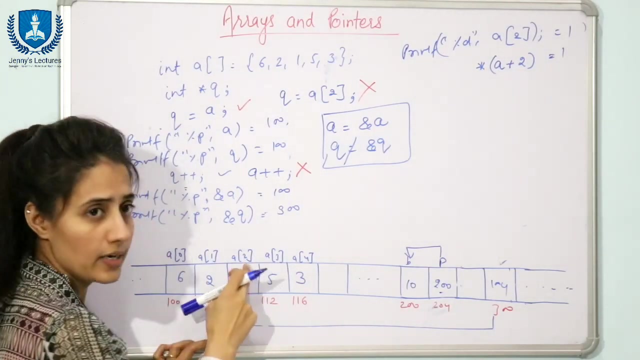 want to print this value, Then what? you will use that d referencing operator, that is s trick operator. so, rather than using a of 2, you can also use this one. this will also give 1. so now, another method to access this variable is using pointers. fine, in this case, if you are, if you have done. 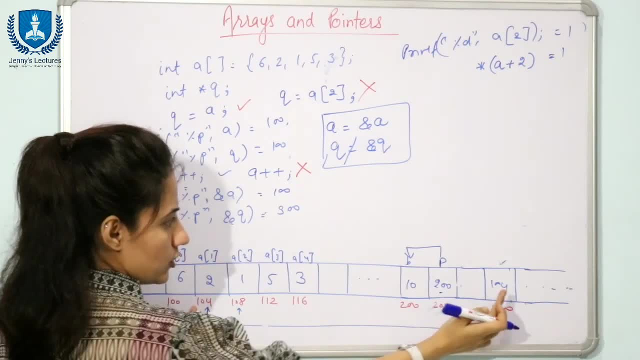 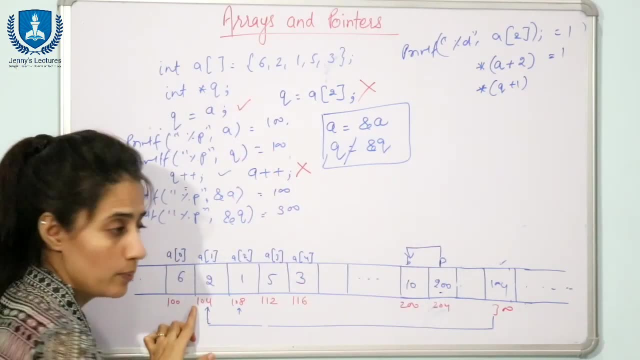 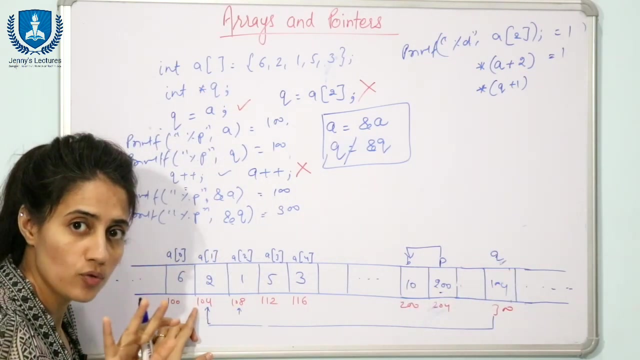 this q plus plus. so pointer is pointing this. now: q contains 104, so you can simply write q plus 1 and s trick because q will contain q contains what: 104 plus 1. if you do, it means 4 bytes would be added. that is 108. and if you want to print what is there at address, 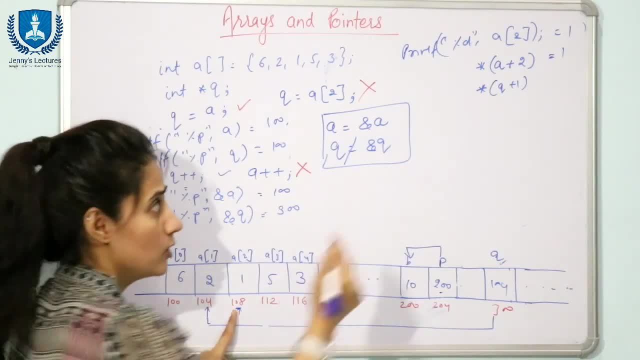 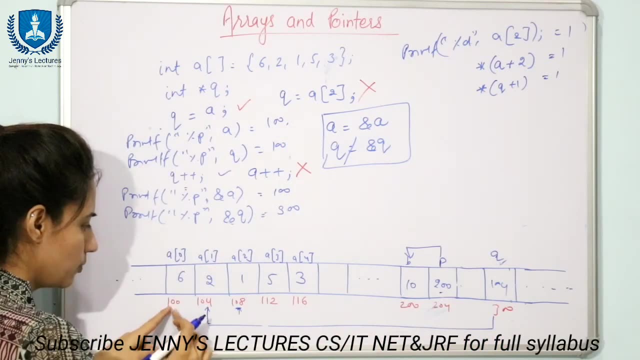 108, then you will have to use d referencing operator, so it will also give you 1. if suppose you have not done this q plus plus and q is still pointing at this base address then you will use s trick q plus 2 and it will print 1.. 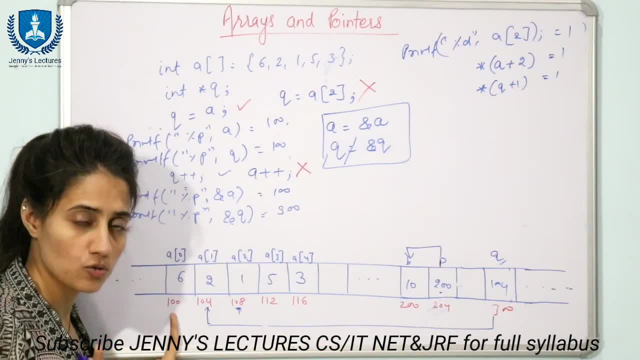 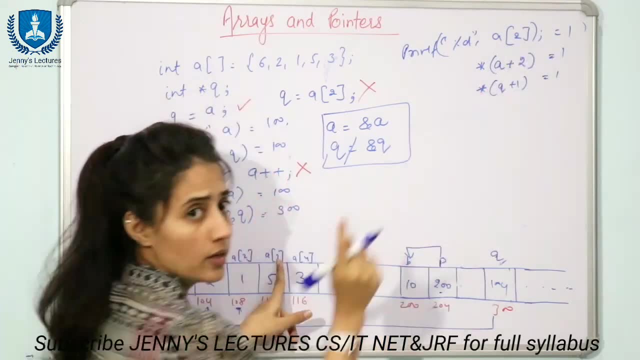 So that is it, And it will print 1, the value, this one, and if you want to print value at this, you want to print a of 3, then simple fundise: you can write a of 3 or you can write s trick: a plus. 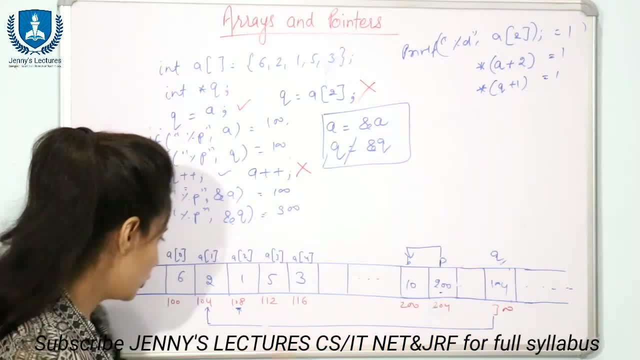 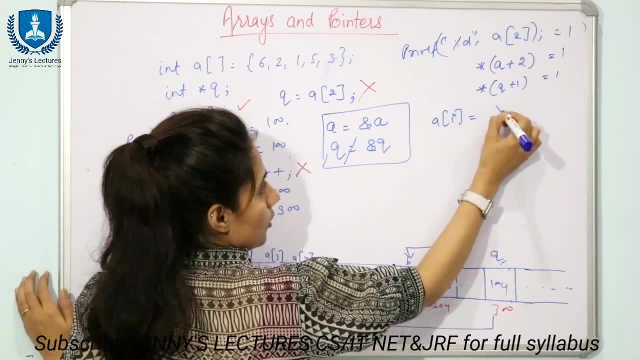 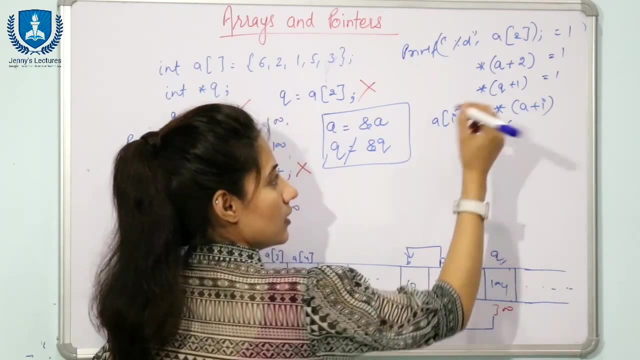 3, or you can write q plus 3 if q is pointing here at the base address. fine. So in another word you can say this: a of i is equal to s trick, a plus i. or you can write s trick. If you are taking some pointers, then also you can write q plus i, because here we are. 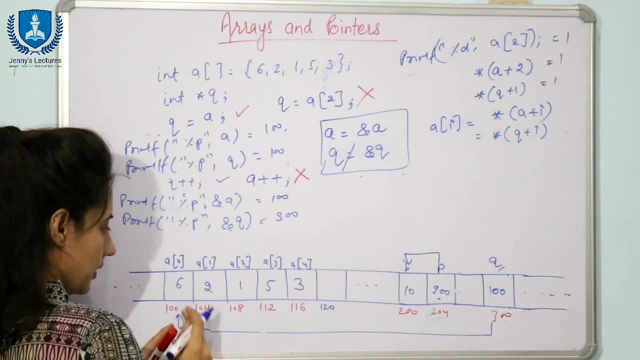 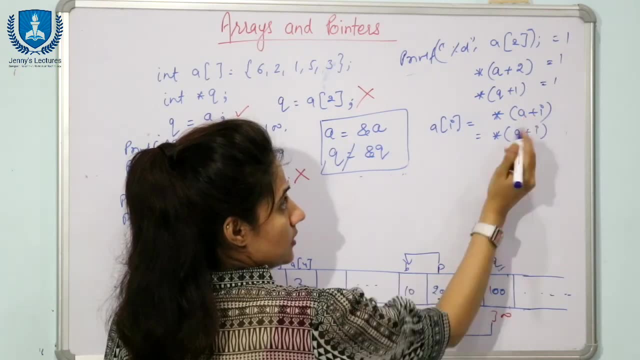 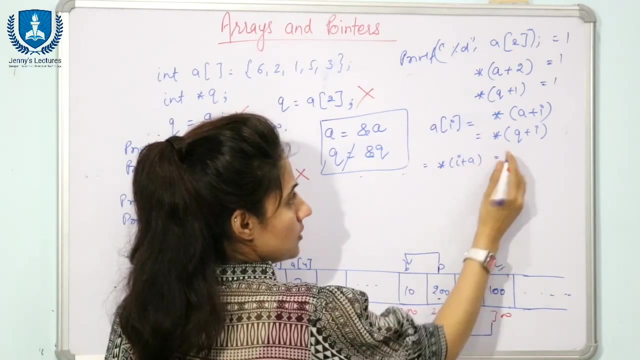 taking q as a pointer, which is pointing toward that starting index of this a, So this is equal to q plus i. fine, now see this: a plus i. I can write here something like this: i plus a, that is also fine, and i plus a, it I can also write here: i add in brackets: 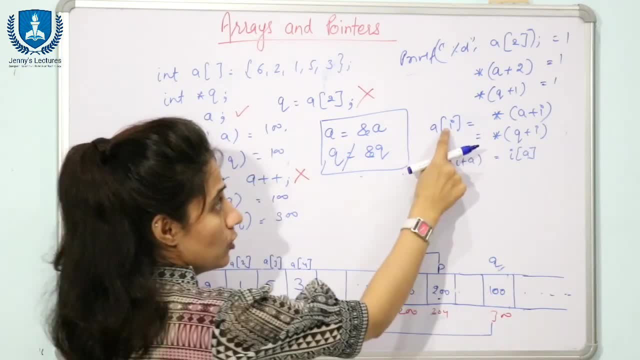 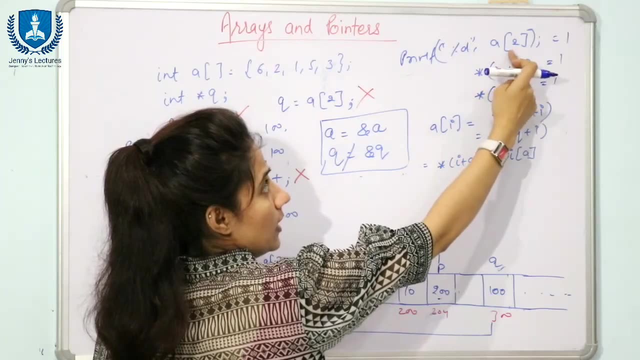 a. that is also fine. So this is equal to this, this is equal to this and this is equal to this right. So you can say, if you want to print value of 2, you can write this also. or you can write 2 of a, that will also print value 1.. 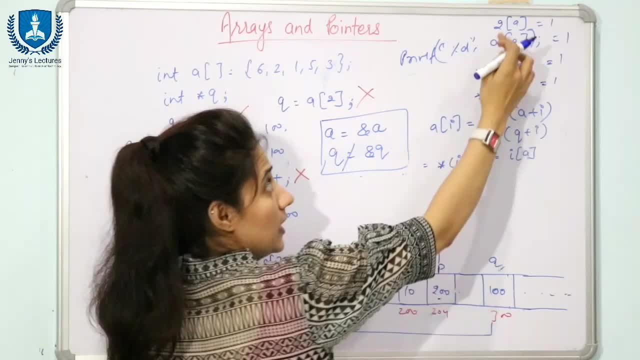 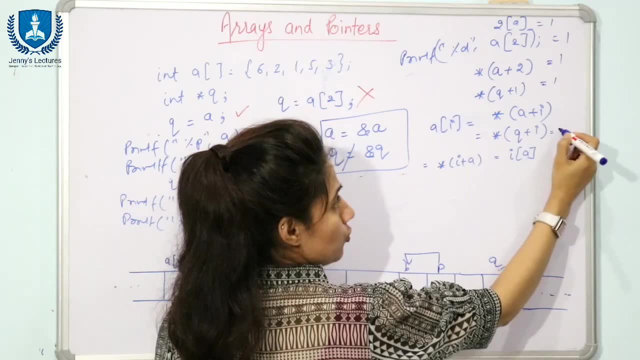 Now you will have to tell me in the comment box: is it printing the same value, a of 2 and 2 of a Next thing, using pointer also? you can print this, so this pointer also you can write here s trick: i plus q. 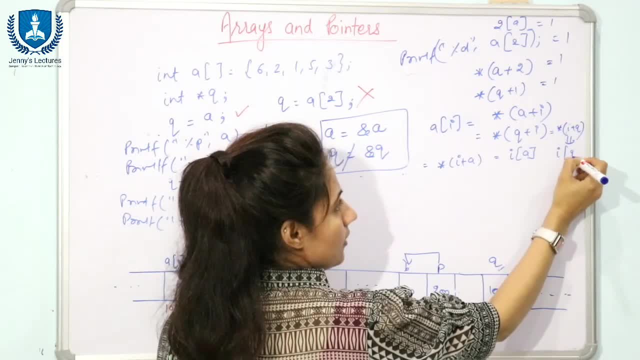 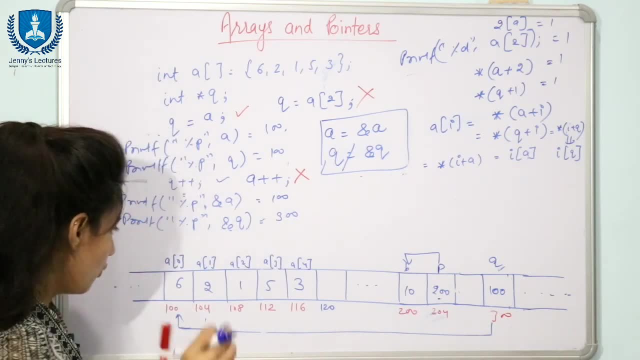 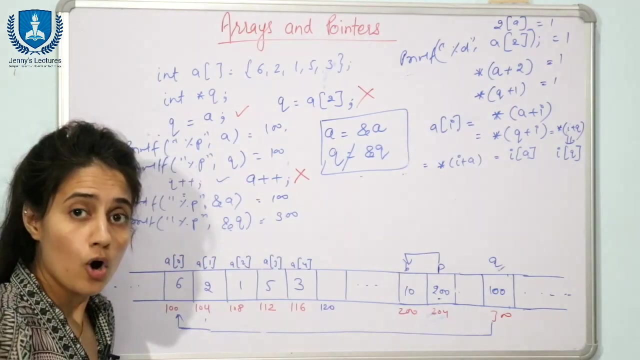 And you can also write i and this q. this is also same. all these terms are same, will give you the same output. Now, next thing is if you want to print the value at this 0th index, then what you will write: percentage d a of 0, fine. or you can write here s trick: a, that will also print. 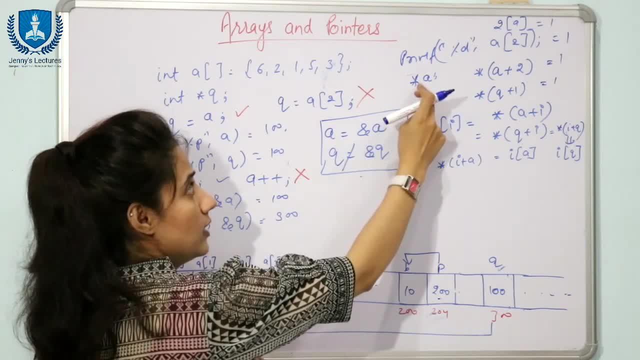 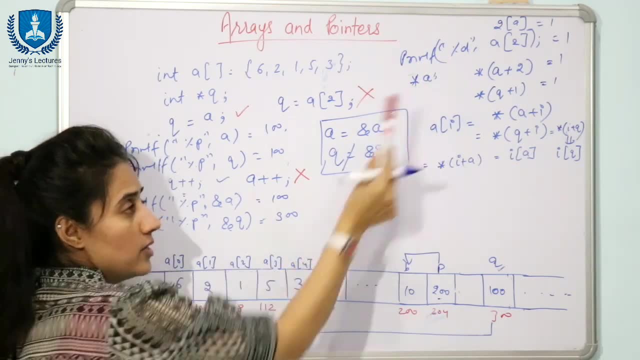 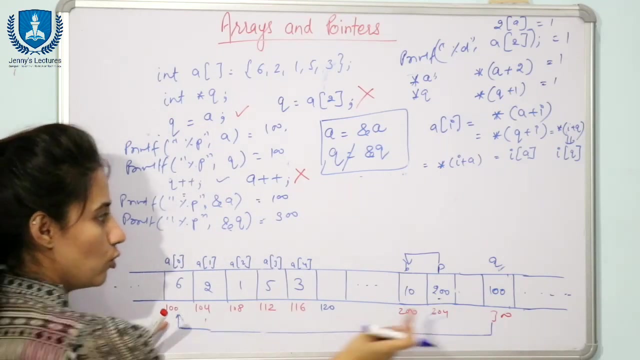 value at this a of 0, that is 6, it will also print 6 a will give address, base address of that array. that is 100 s trick means value at this address. value is 6, right? or you can write here s trick q, because q is also pointing here. q also contains 100. 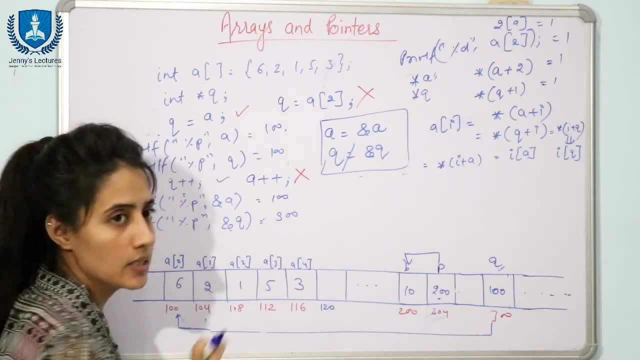 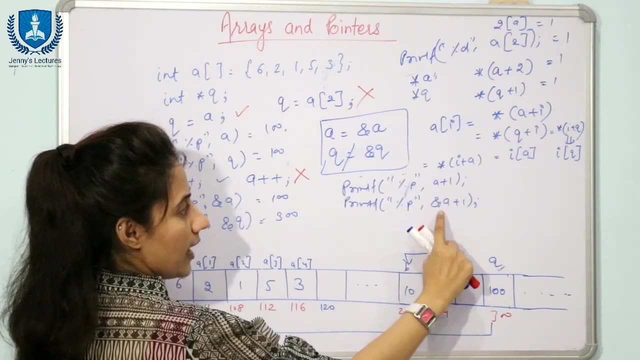 So value at 100 is 6.. So it will also print 6. fine, Now next thing: if you write see a plus 1 and address of a plus 1.. Now what should be the output of these 2 lines? a plus 1.. 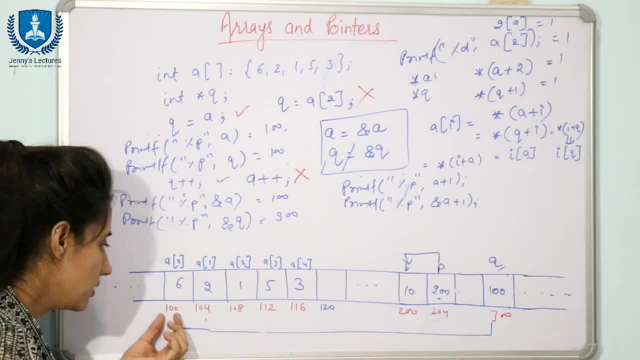 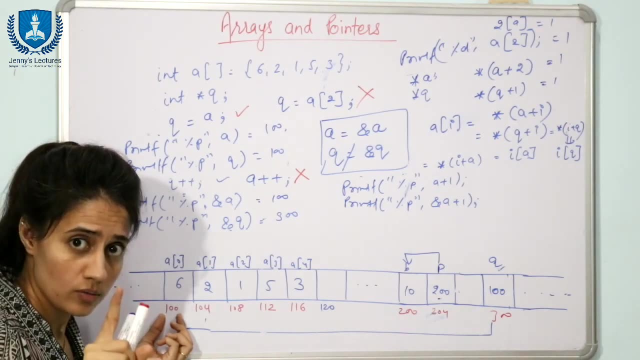 a means it will. it contains the base address of array, that is 100. if you add plus 1 in 100, it will point to the next element address. it will not give you the value 1, 0, 1 in this case, because I am considering base address 100. actually it should be in hexadecimal form. 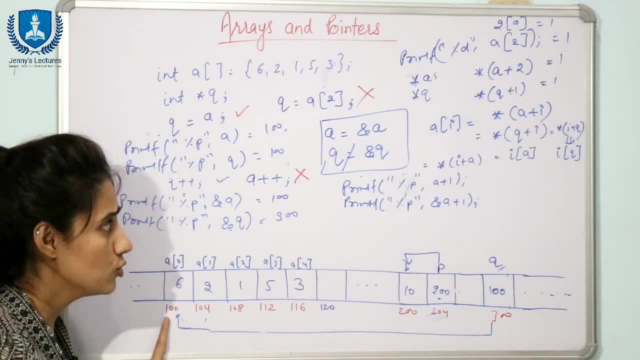 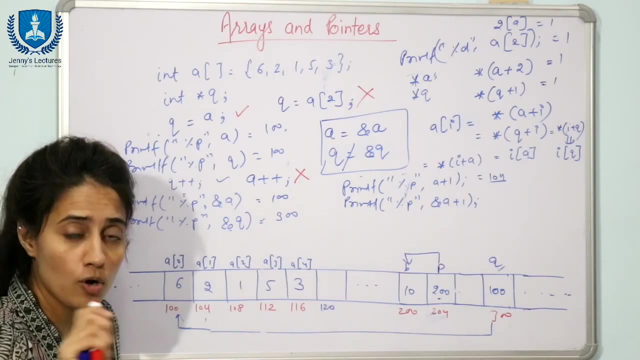 I am using this percentage p. fine, So it would print 1 0 4 plus 1 means the data type is integer. integer will take 4 by its. that is 1 0 4, and if you print this one address of a plus 1, it will not give you 1. 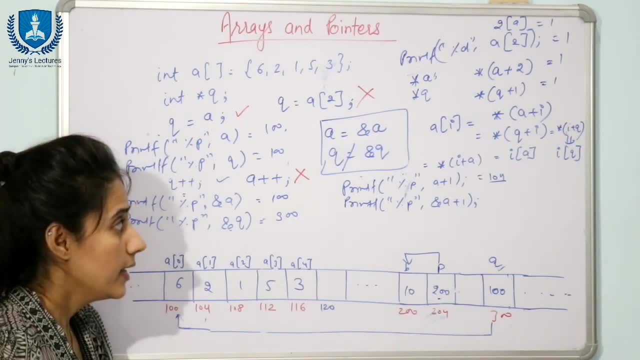 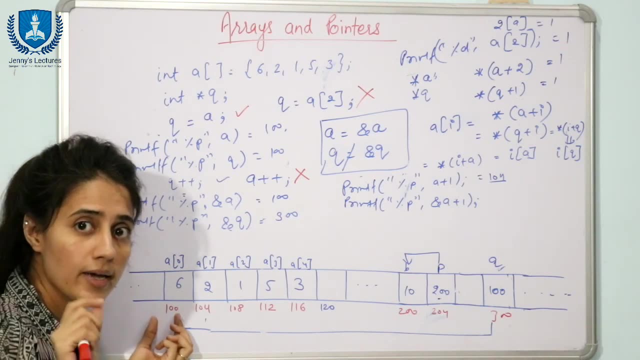 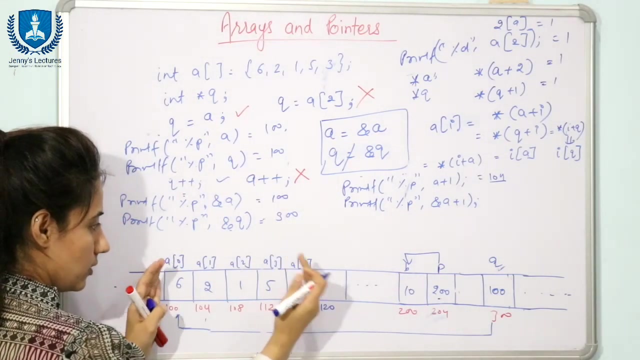 0, 4.. Now what should be the output of this one address of a? obviously, address of a and a is same. address of a means 100, and if you want plus 1 in address of a, then it will increment it by the. you know, with the, the complete array address. 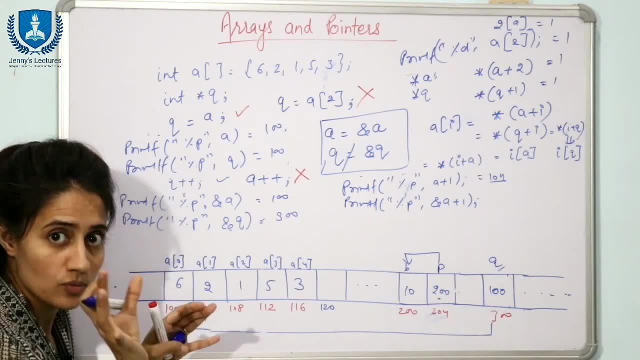 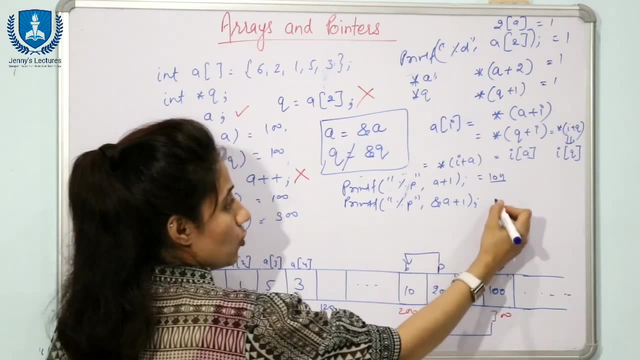 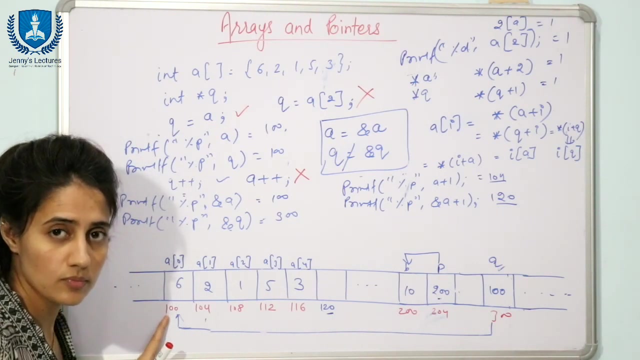 So complete array contains 5 elements. Okay, The address for I mean the size of 5 elements would be 5 into 4, that is, 20.. So it should return 120. in this case It means it will point to here 120, fine. 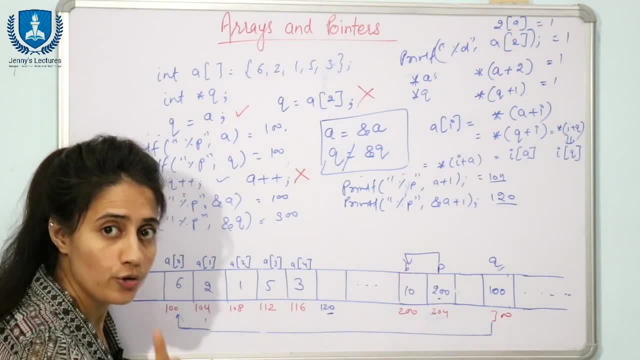 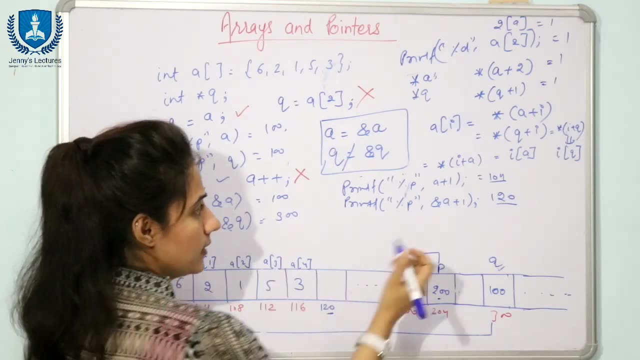 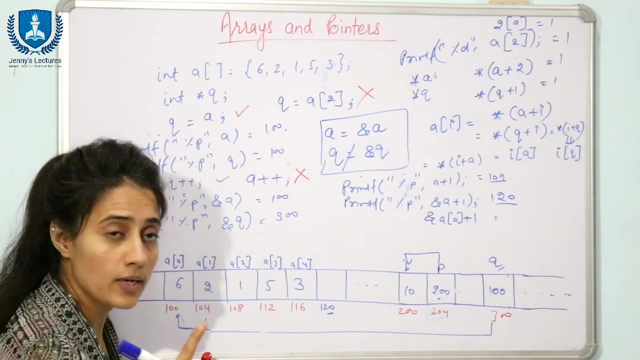 So these are 2 different things. Now I want you to execute these lines and tell me: is it following the same logic or not? and now, if you print address of a of 0 plus 1.. Then what should be the answer? that should be 1 0- 4, because address of a of 0, specifically. 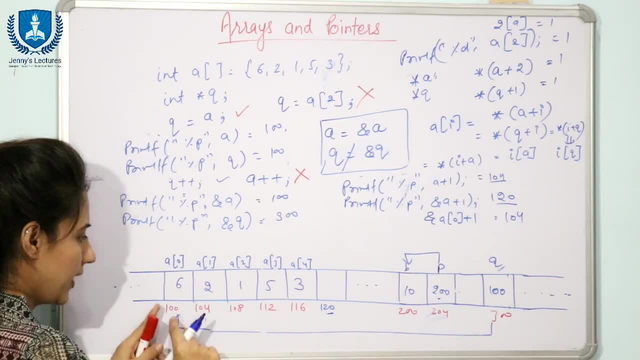 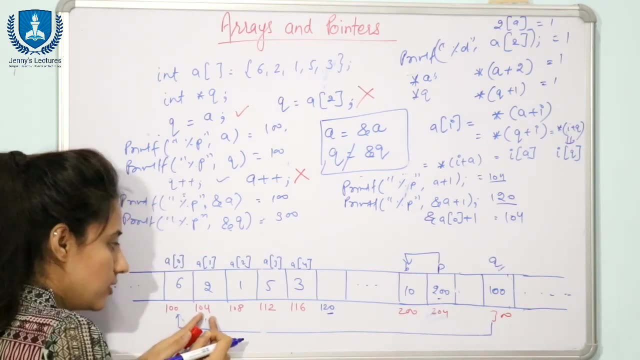 you are assigning a of 0. a of 0 means this one address is 100, and 100 plus 1 that is 1 0, 4 first element: address plus 1, that is this one only. but if you write simply address of a plus 1, that could return 120.. 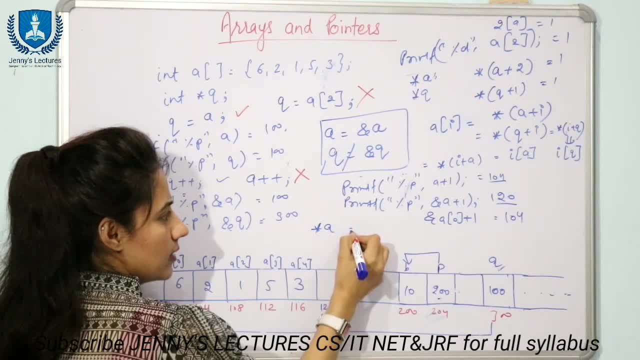 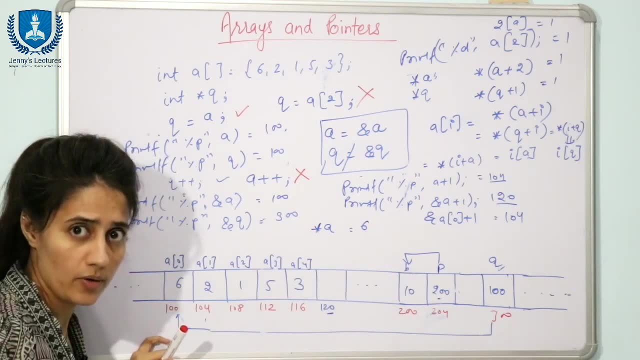 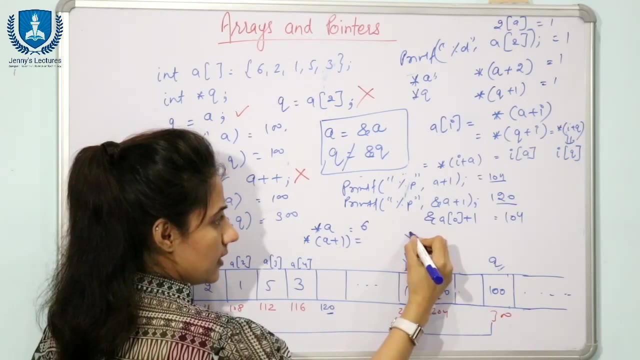 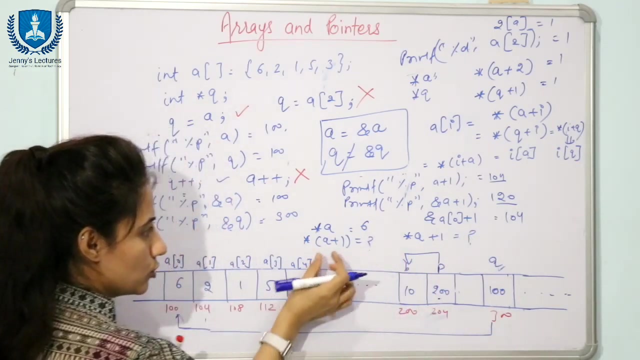 Now, if it in printf, if I write asterisk a percentage d, asterisk a, then it will print what value at this one it means 6, it will print 6, right. and if you write asterisk a plus 1 and another thing is asterisk a plus 1, these 2 outputs see. here I have used brackets. 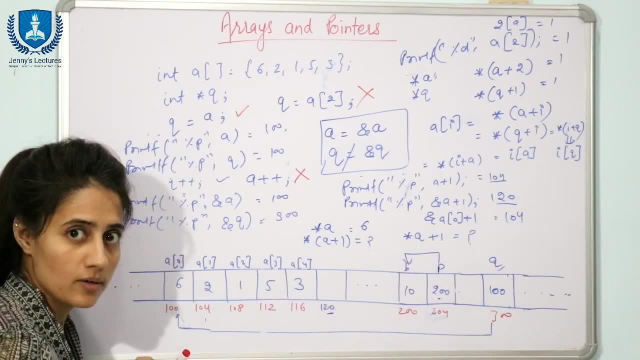 here, I am not using brackets. Now, in the comment box, you are going to tell me what should be the answer of this one and what should be the answer of this one. Fine, I am leaving it up to you, because I have discussed many things here. 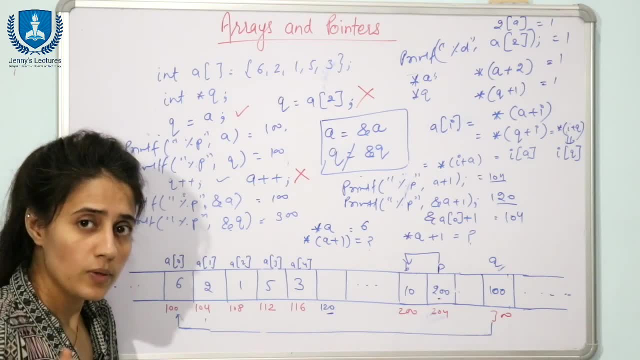 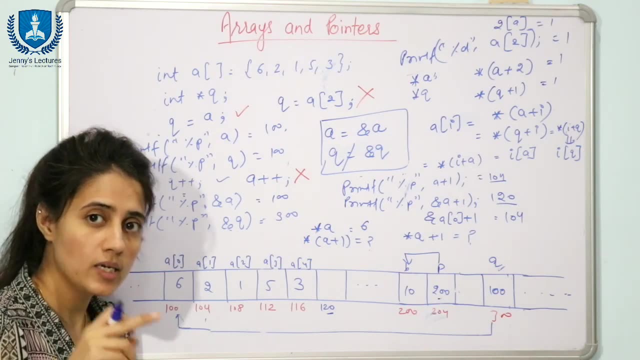 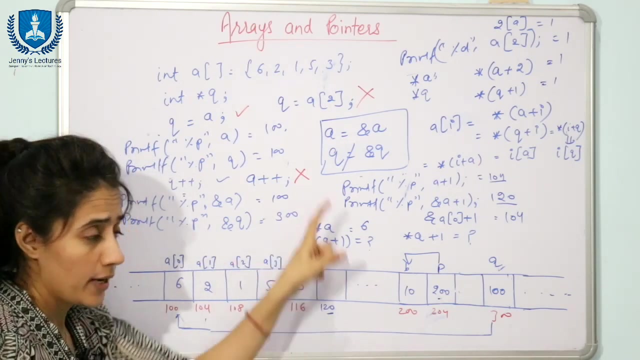 See, I cannot discuss everything in one video. so simply, if you want to, you know, grab the concept and if you want to remember the concept for a long amount of time, then the practice is a very good thing in case of programming. So I am again and again saying: just do practice of these things. I cannot tell you everything. 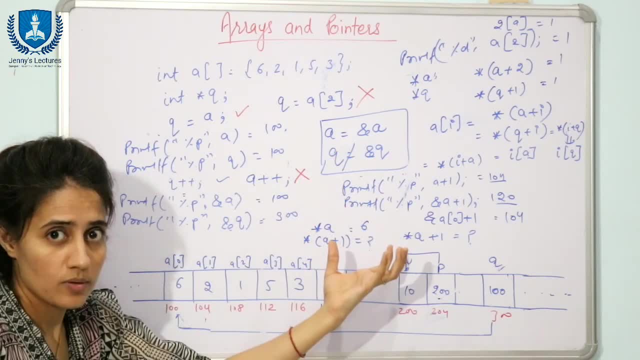 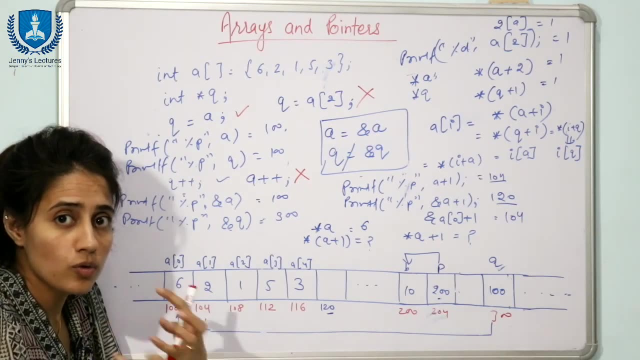 so just try to modify these things also. fine, See, I have told you that I can write q plus plus. so it is up to you that you have to, you have to be a critical thinker, you, you have to try that. can I write q into 2? can I write? 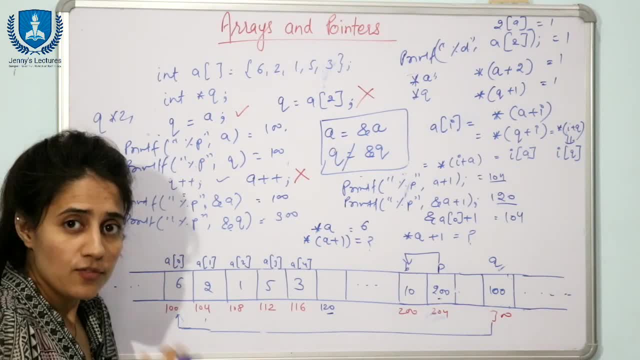 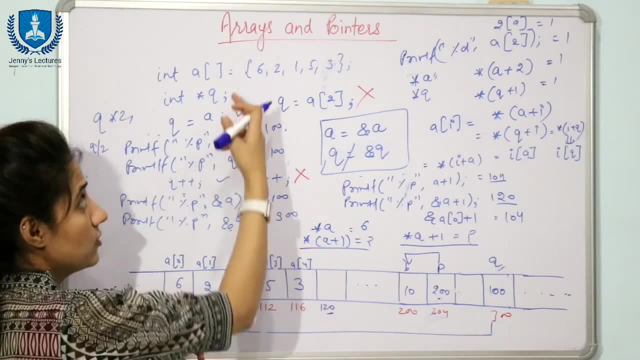 q divide by 2, something like this. and if you do practice a lot of practice, then you can easily grab these programming concepts. See, maybe you will initialize this array with some other values and you will get some value here. and you will get some value here if you will not get why you are getting these values. 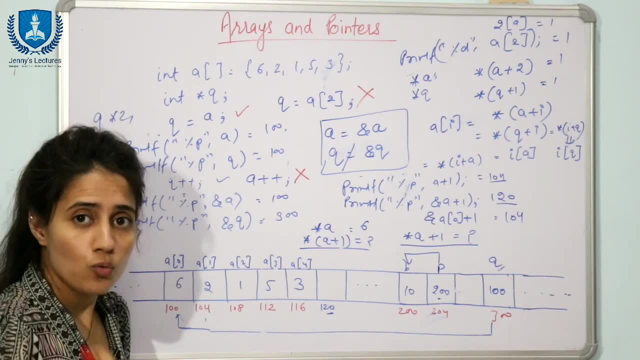 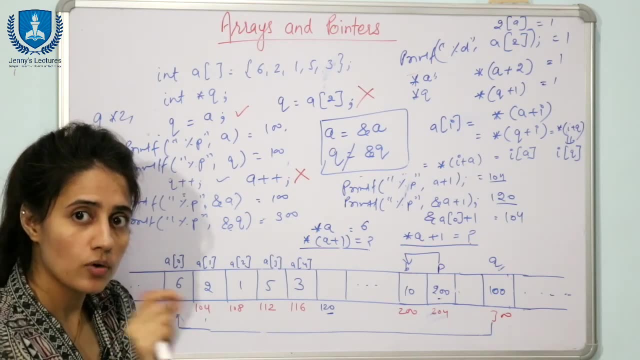 here, then you can ask me in the comment box. Now I am going to write a simple code in which we are going to initialize the array at runtime only and we are going to print that array using pointers, not array. So here I am, taking one array- size is 5, declaring one array. I will initialize the array at runtime. 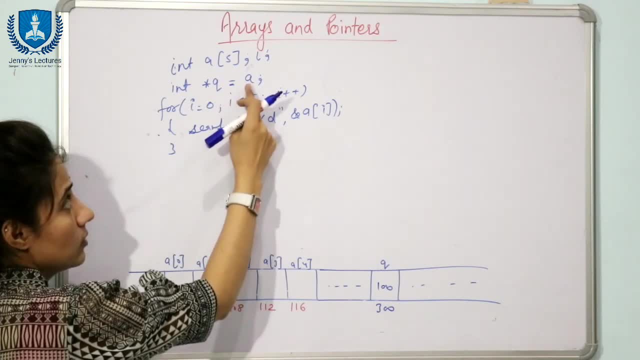 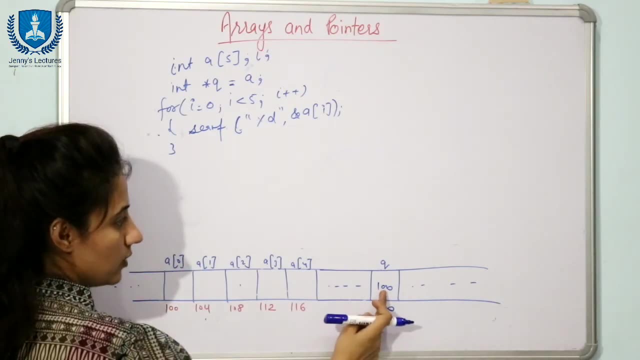 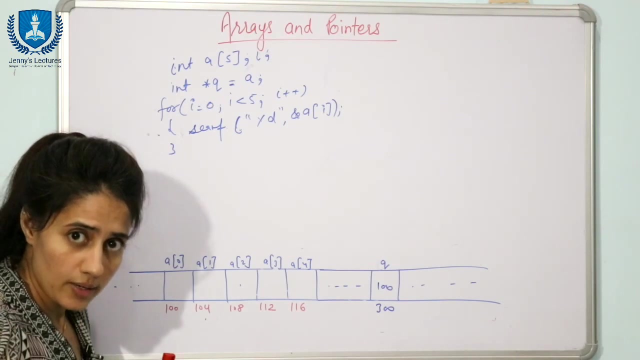 one pointer I am taking. that is q and this q is containing address a. a means it will return the base address of array, that is, 100. it will. it will. it will contain 100, and suppose the address of this q is 300. now I am going to take input from the user, so one for loop. 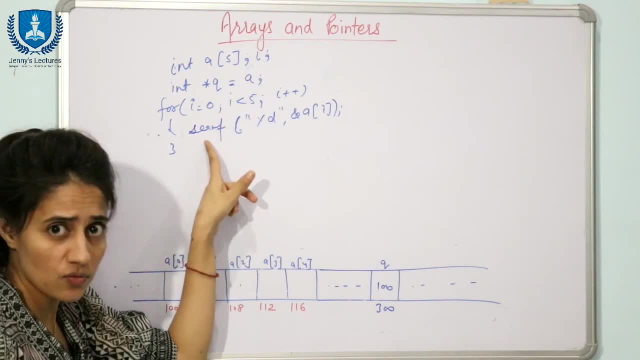 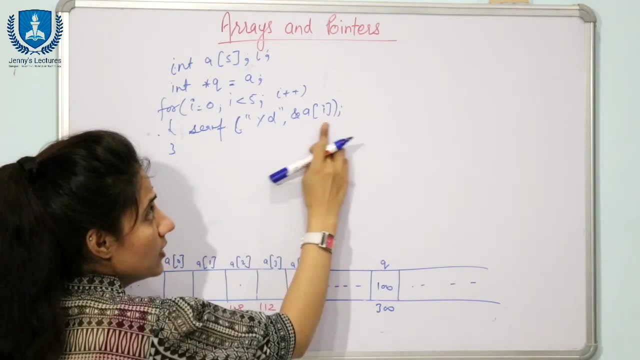 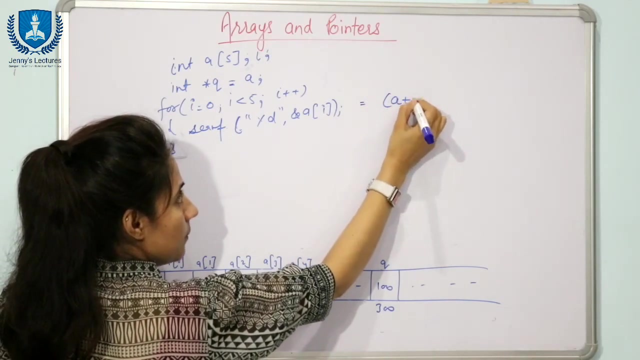 would be there from 0 till this size i plus plus. scanf is a function which is used to take input percentage d, and here I am writing address of a and i in this case, in this case, I am writing this case, this one, and at this place also I can write a plus i rather than. 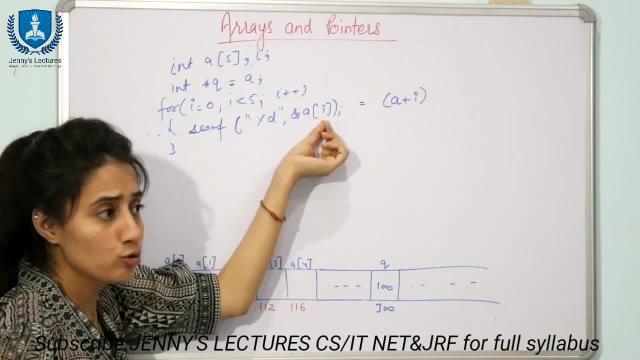 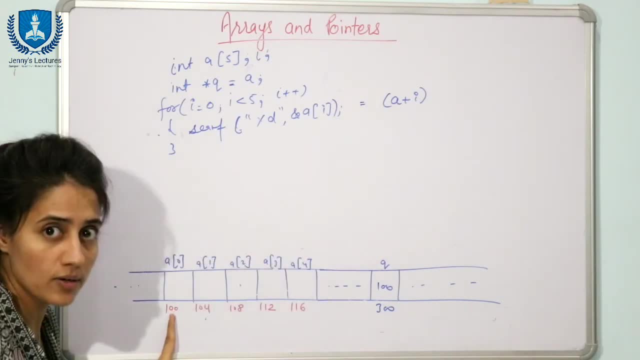 rather than writing address Address of a of i, you can also write a plus i, simply a plus i, because see a will return address: 100. in first case i value is 0, 100 plus 0, that is 100 only in second case i plus. 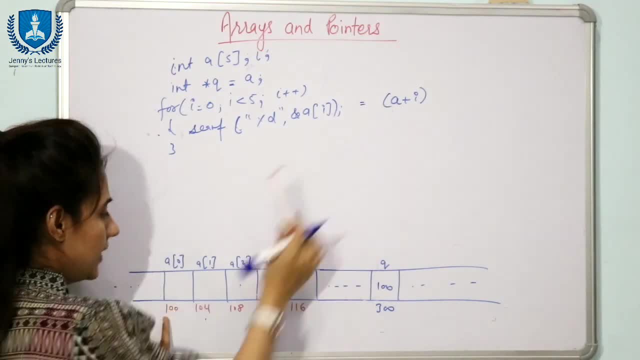 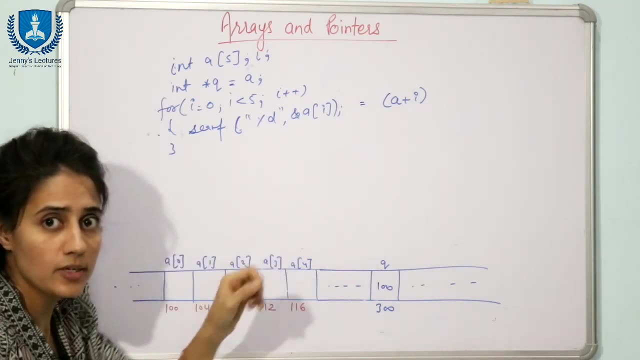 plus i value would be 1 a plus 1. that means a contains 100. 100 plus 1. 100 is a point address and it will. if you add plus 1, it means it will contain the address of next element, that is, 104.. 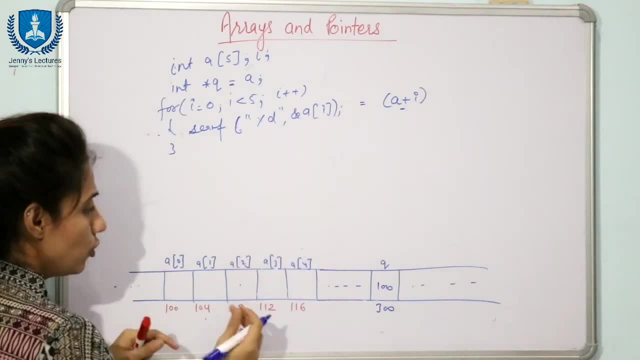 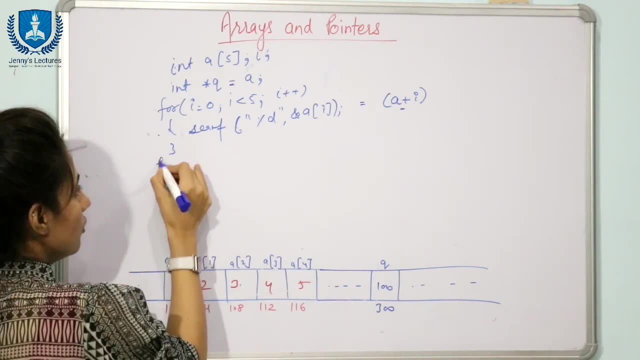 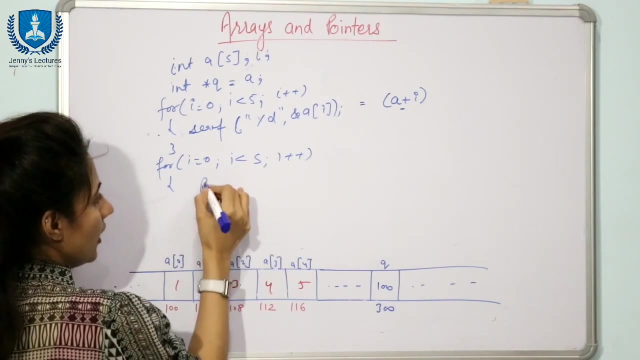 So you can write this also if you want to print now value. suppose user has entered some value that is 1, 2, 3 and 4, 5. now if you want to print these values, then another for loop would be there, from 0 to less than 5 and i plus, plus. now I am going to print the values. 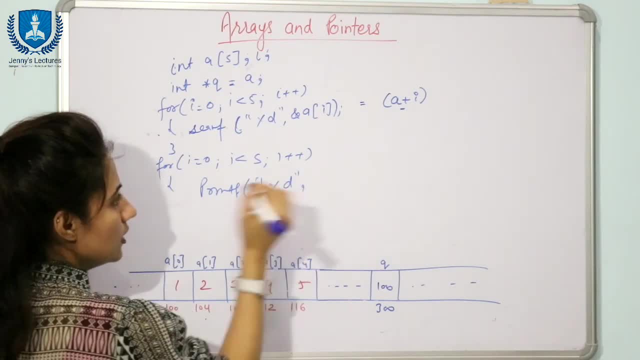 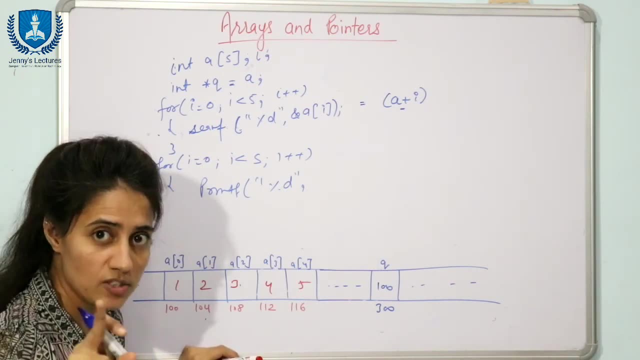 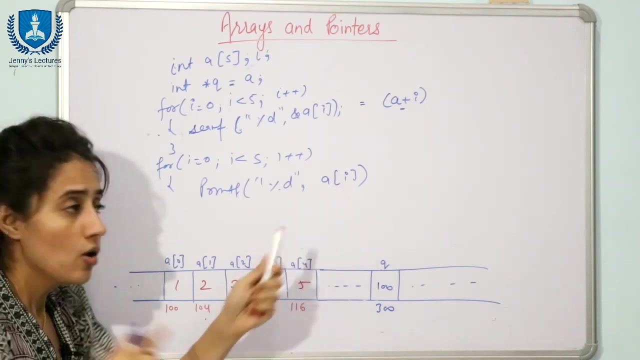 using pointer. so how you can print these values using pointer: see using pointer. if you want to print, then you are going to use simple dereferencing operator. here you can print a of i also. simply, that means you are accessing the value of i or rather than writing a of. 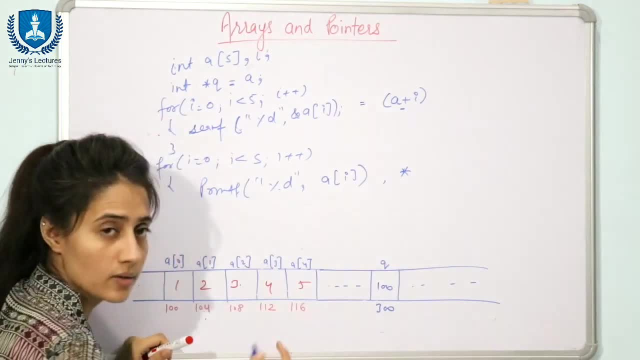 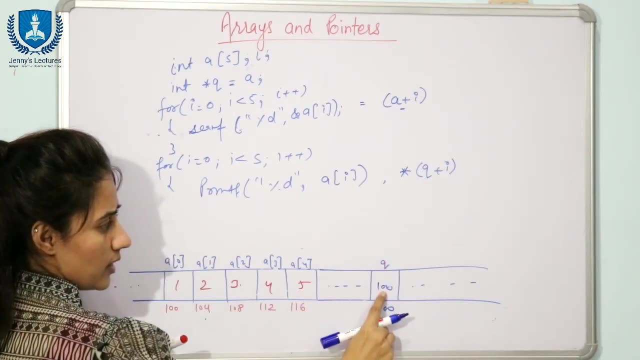 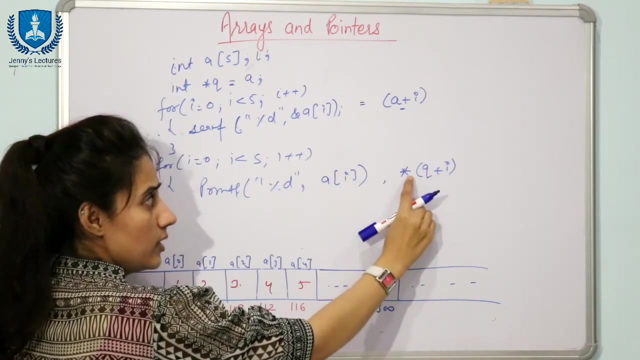 i what you can write asterisk: q plus i. that is also fine. q means it contains base address, that is 100. so 100 plus 0 at first iteration. 100 plus 0 means 100 only asterisk means it will print value at this address. value at 100 is 1.. 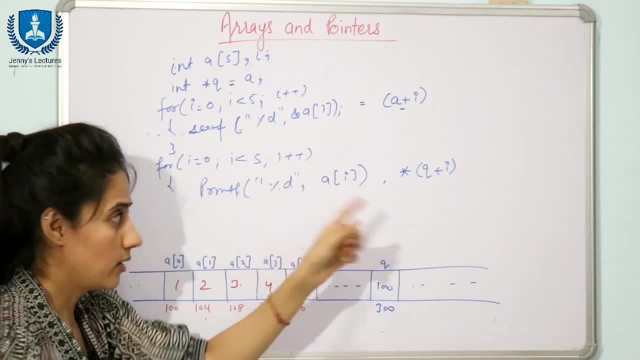 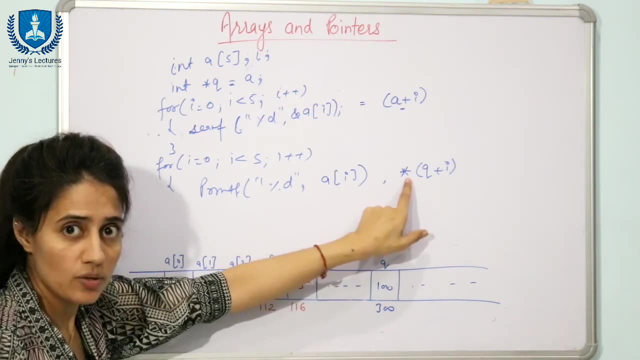 Next time i would be i plus plus, that is 1. it means q plus 1, 100 plus 1. it will point to the next address: 104 asterisk means value at 104, that is 2. so it will print 2, so like: